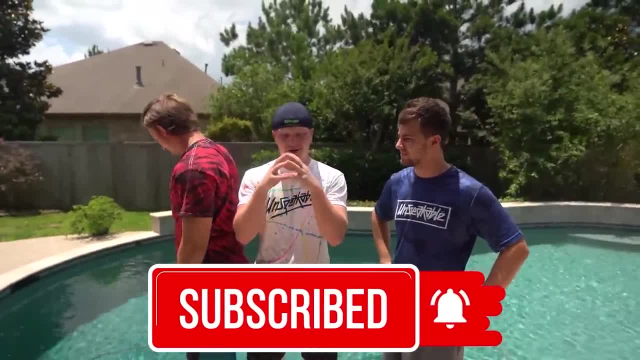 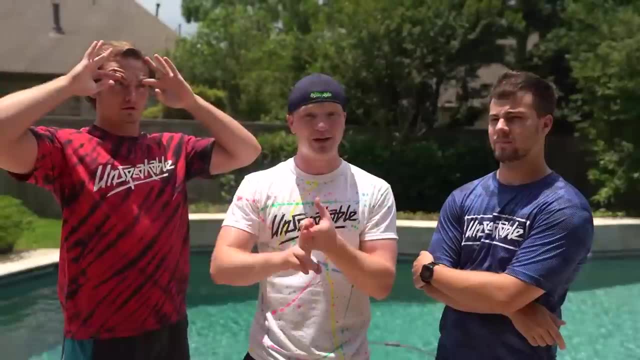 because today we have something so cool for you guys, Something that is so indestructible and so strong. It's stronger than titanium. It's a material that is used for aircrafts, spaceships and even missiles. You can literally drop it on a car and it can destroy the car. It's insane. 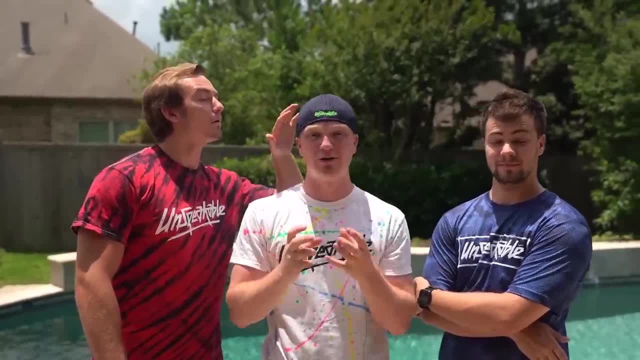 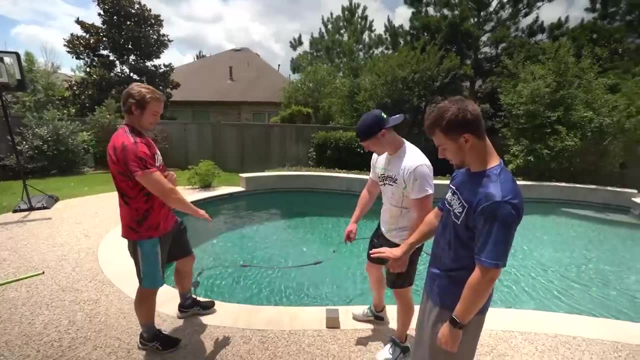 Very happy. I am so excited. This cube is also indestructible. It is almost as strong as diamonds. It's actually right here. Look how tiny it is. Look at it. Look how tiny it is. It's very shiny. 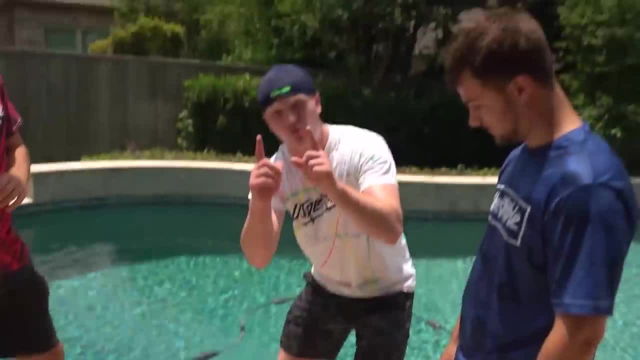 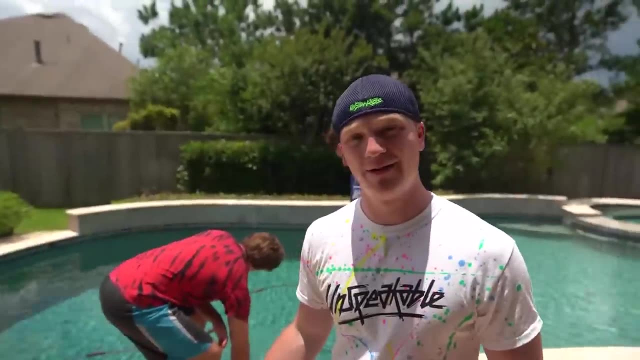 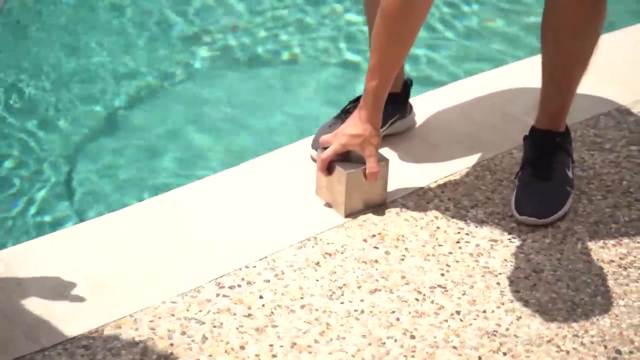 So this cube is 45 pounds and it's only four inches big. Before we get into destroying things with this cube and trying to destroy it, we're going to try to pick it up and show you guys how heavy it is. Try to pick it up with one hand. You need two hands. You can't pick it up with one. 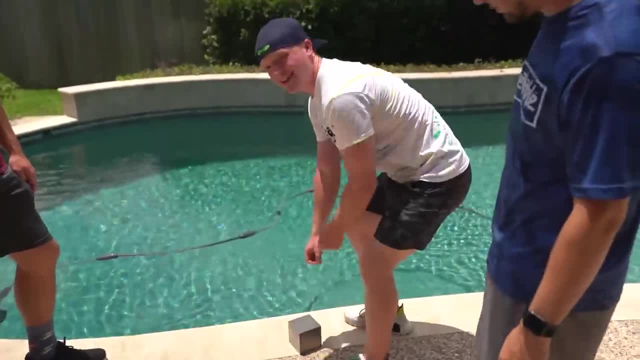 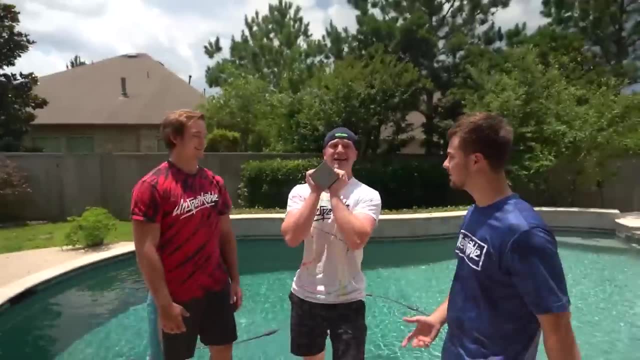 hand. You just can't. It's got like crazy grip, Literally impossible. I don't think you guys realize When you pick it up and you feel the weight, it just doesn't make any sense. Okay, It's so heavy, So this cube is very heavy, It's. 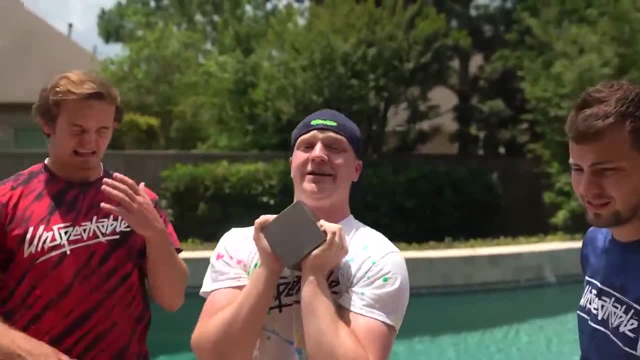 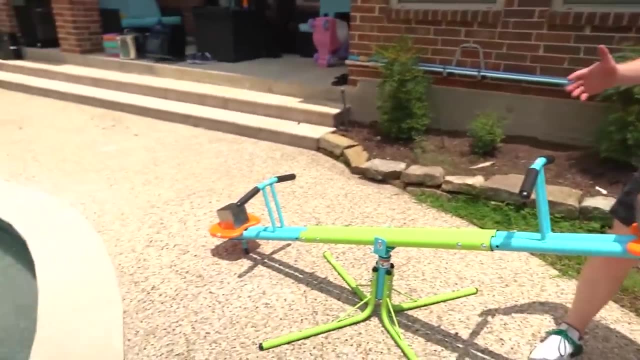 bulletproof. It's indestructible. Let's show you, guys, how heavy this thing is. We have the cube on this side of the seesaw and this is a really heavy kettle weight And, as you can see, it's not even budging, Literally doing nothing. Push it down. Push it down on that side. Okay, Got it All right. 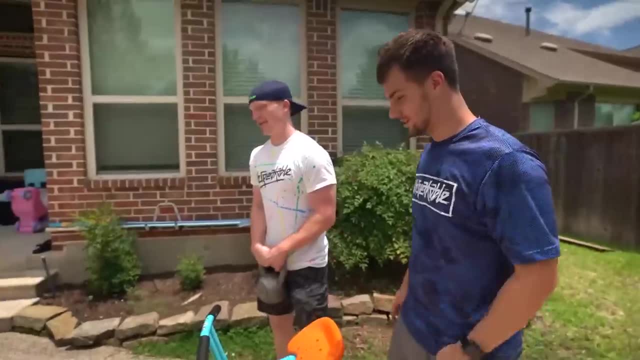 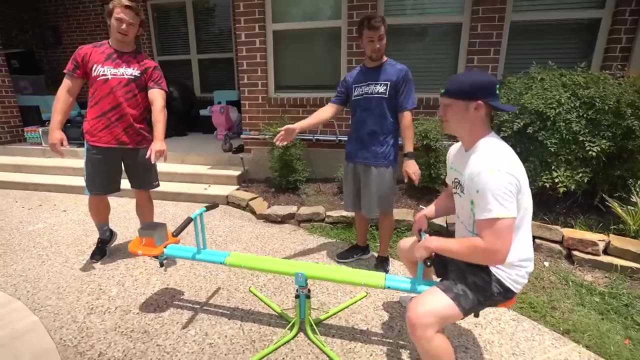 You ready? Yep. So the cube wins that round. You can literally use it as a seesaw weight. If you don't have any friends, buy this cube so you can seesaw. It's literally half the weight of me And you know what? It never talks back to you either. 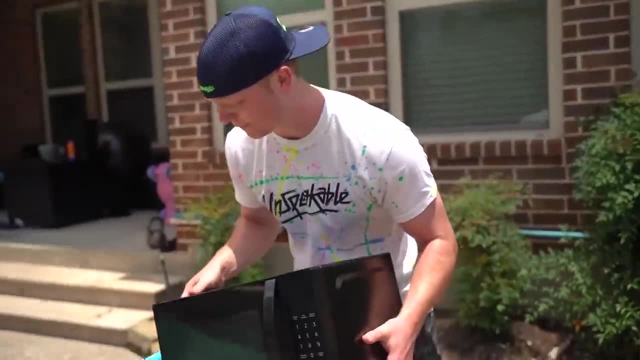 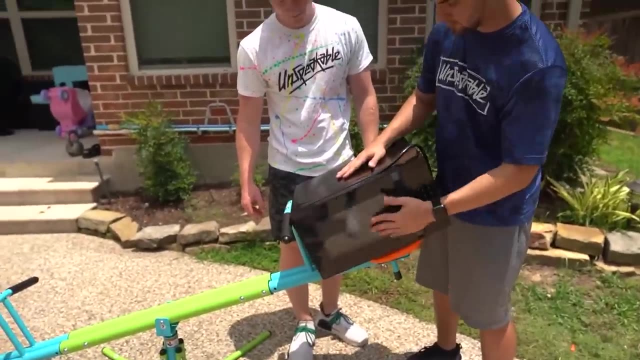 It doesn't. It doesn't talk at all. So now we have an entire microwave. Wait, hang on Nothing. Oh, you didn't plug it in. Oh yeah, You got to plug it in. Plug it in: The microwave looses the space. 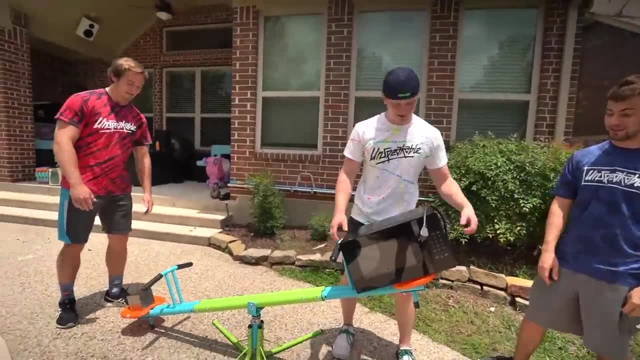 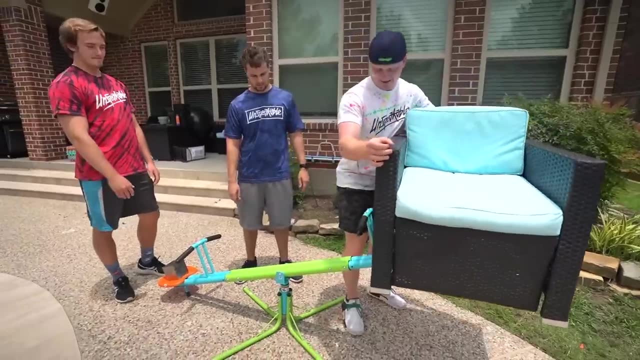 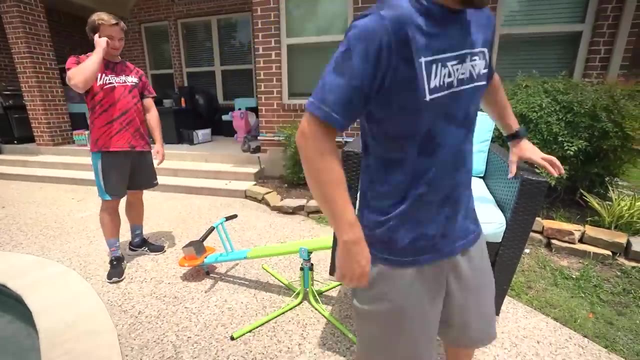 You still need like a decent amount of weight. Okay, Maybe we should do a fridge next. I think we should do a car. Now we have an entire chair. You still didn't move it. As you can see, it's still heavy. Maybe you should sit on it. Gabe, I don't want it to go in the pool because if it, 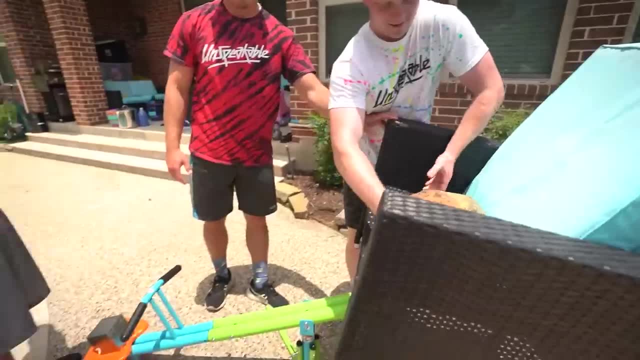 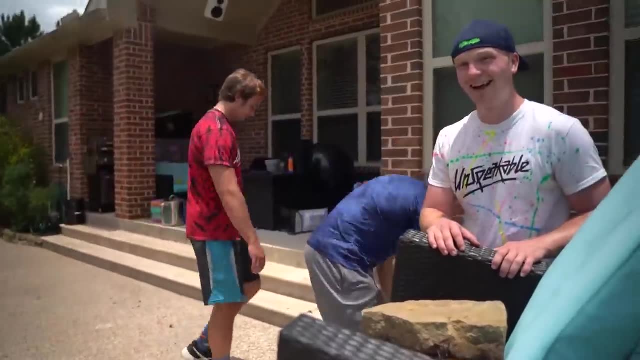 goes in the pool. we're not getting it out. Let's give this chair a little bit more weight. Nothing, Another one. Nothing. Give me another rock. Okay, Rock number two. There's some big rocks too. Nothing. Rock number three. Oh, there it is, Three rocks and a chair It might balance out now. 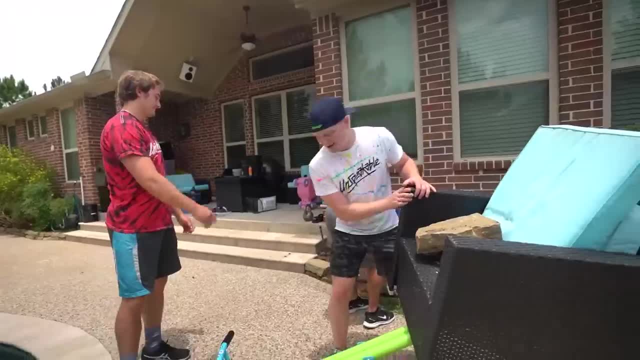 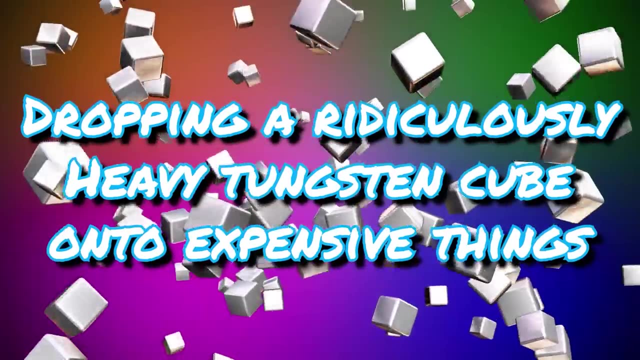 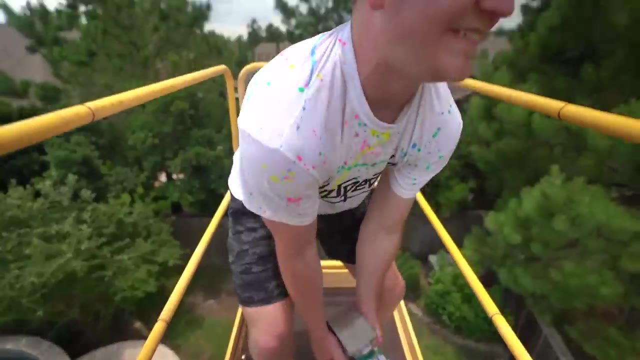 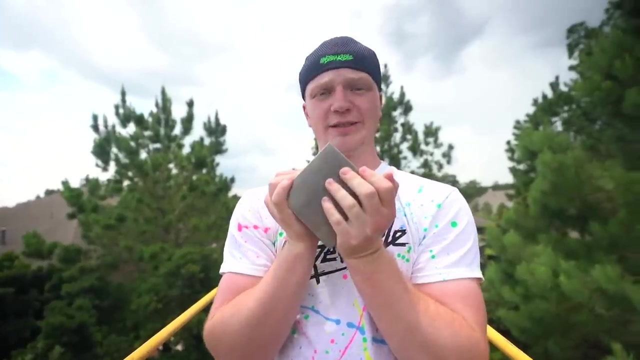 It's winning. It's winning, Oh, Okay, So you get the point. The cube is really, really heavy. Now let's drop it on some expensive things, Okay. It is insane how small This cube is and how heavy it is. That's what amazes me. If you had two of these, or two and a half of these, it would literally be as heavy as my entire body. 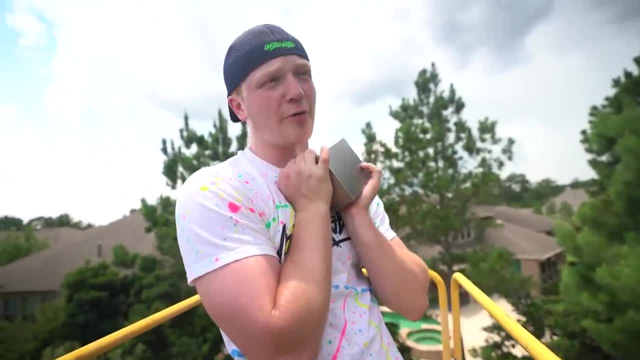 Our first item that we're going to drop it on. It's kind of exciting. It is going to be a microwave, but not just any microwave. This microwave is cooking up some popcorn. Well, we got a microwave, We got some popcorn. We have an extension cord. 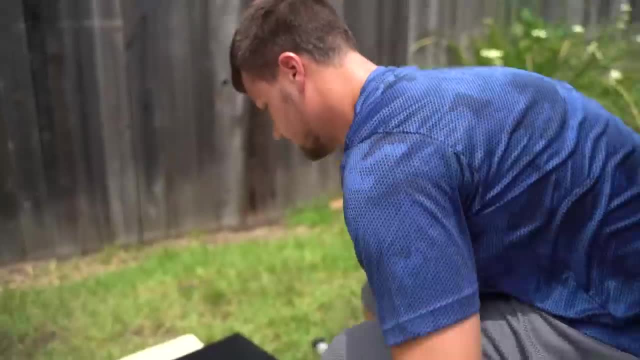 Throw it in there. Throw it in there, Hit popcorn. All right, it's going Move it a little bit closer. How am I going to make this? I hope I don't miss Same. Yeah, the, please don't. 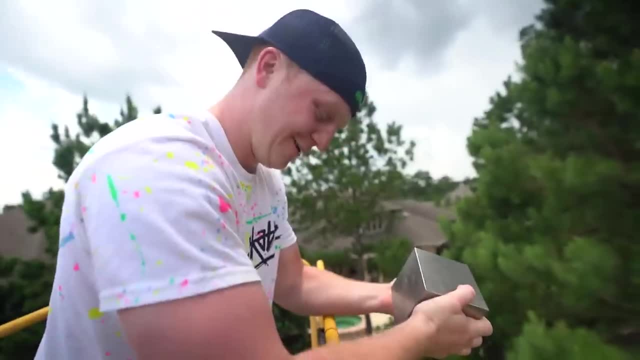 Let's popcorn cook a little bit. I guess I can't do this thing. It's literally going to outweigh it. It's literally going to outweigh me and flip me over the edge. All right, whenever you're ready. All right, ready. 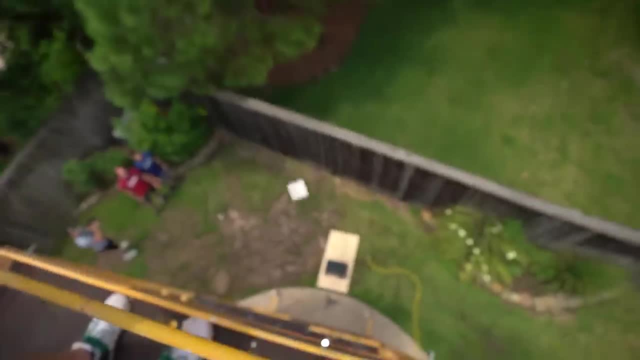 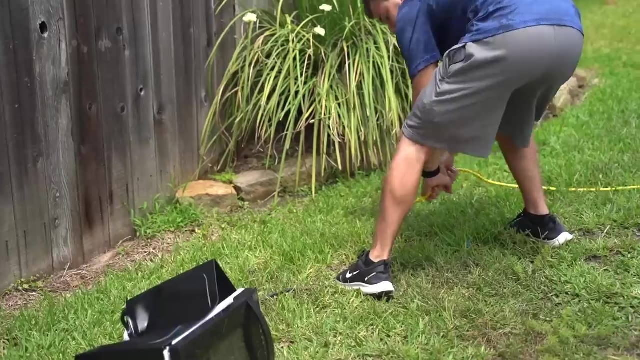 Yeah, Three, two, one. He's going to miss it. Watch him miss it. He's going to miss. Oh man, Cool Destruction. Well, no one's cooking popcorn in that microwave anymore. Wow, That microwave will never work again. 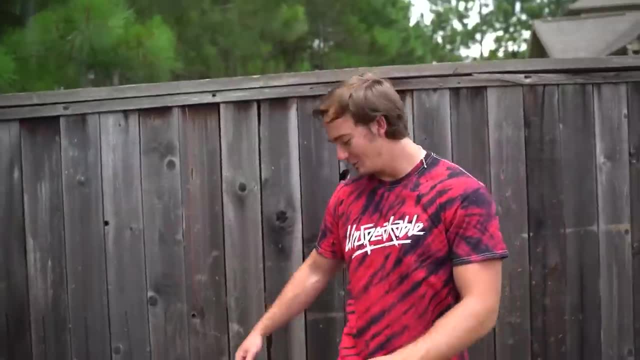 Check the damage. Check the damage on the cube. What damage to the cube? The cube even has a scratch on it. It's got dirt on it. but that's about it. Yeah, it got dirt. Do you want to try it out too? 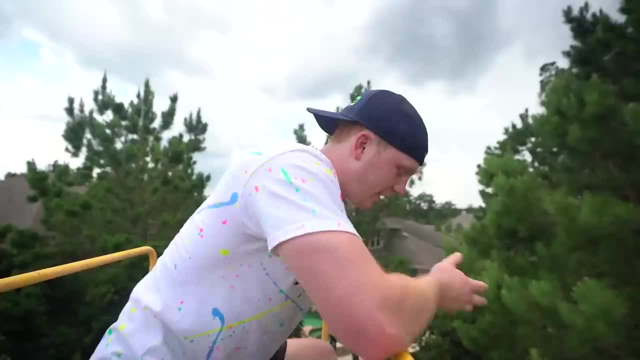 The cube just has dirt on it. That's it. Wow, You want to try it again, Maybe on the face? Yeah, like flip it up. Okay, so we're trying to get the cube up here efficiently. I wouldn't even use the pole. 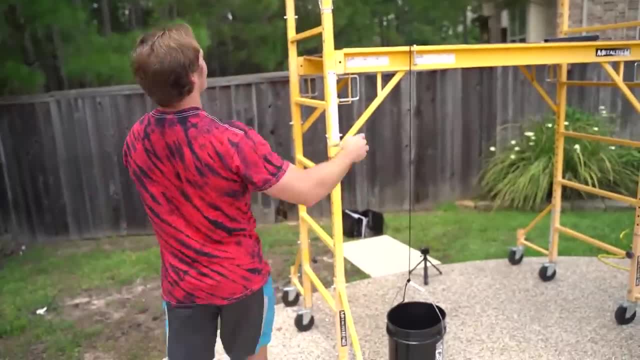 I would just pull it. Yeah, like that, Like how you're fishing, Dude, this thing is so heavy If you wrap it around the other bar, kind of like a pulley system. it should make the load a little bit lighter. 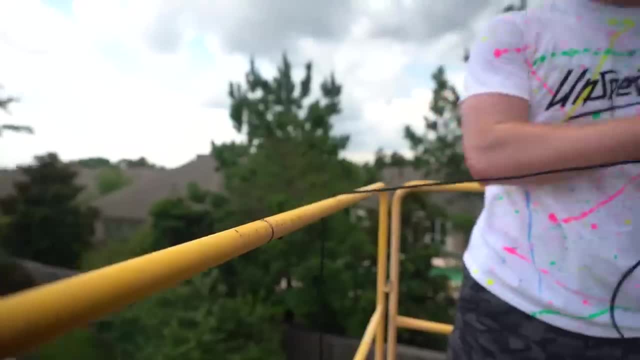 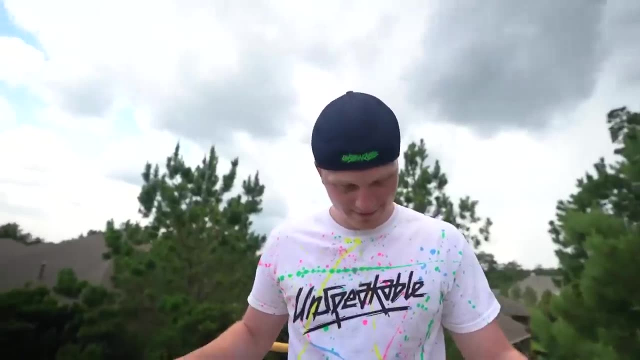 What if someone from the other side pulled down on it? Yeah sure, I literally can't even lift it up. Watch that whole rack up there fall. What if the scaffold flips? No, just those guardrails. All right, I'm ready to do my part. 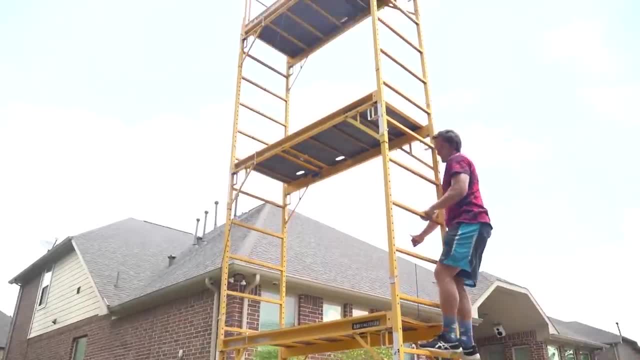 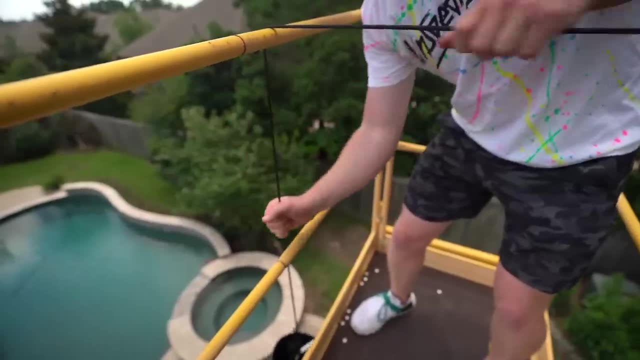 Go for it. Okay, we're doing it. We're doing it. We've got two people pulling up this one cube. Oh, there it is. Oh No, Hold on, hold on, Keep pulling, keep pulling, Swing it. 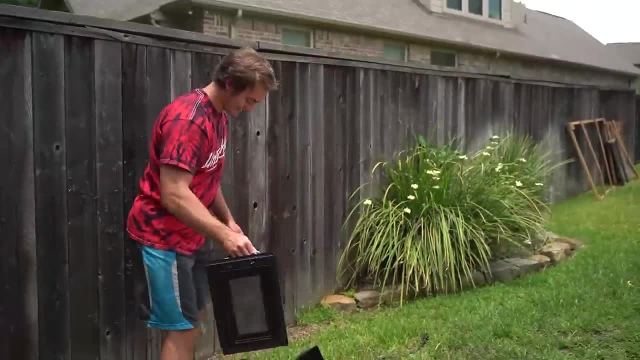 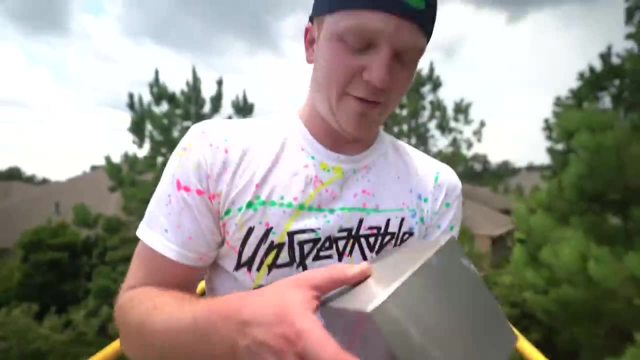 All that just for this one cube. Oh man, popcorn's not even cooked. Put the lid on it. Hey, which way does it go? Yeah, Drop number two on the microwave And, as you can see, literally that's the only damage I see on the cube. 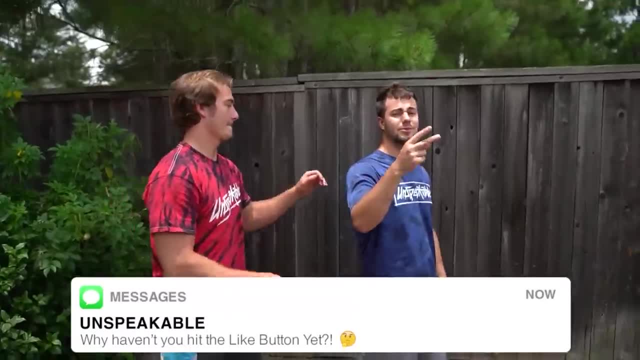 That, and it's probably just paint from the microwave. All right, here we go. All right, here we go. Round two on the microwave. Oh, am I gonna be down? Yeah, I'm just gonna give you a massage, bro. 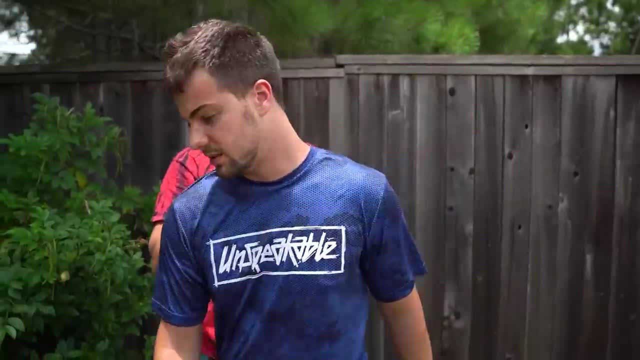 I feel like a body shield. Yeah, there's kind of no, just a massage. Let's just back up a little bit. No, no, That's good, I wanna see it. Drop that cube. All right, here we go. 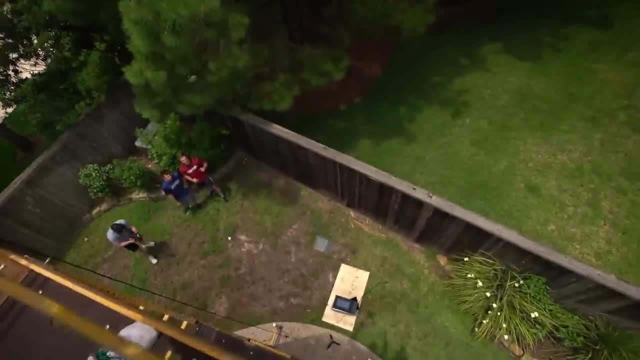 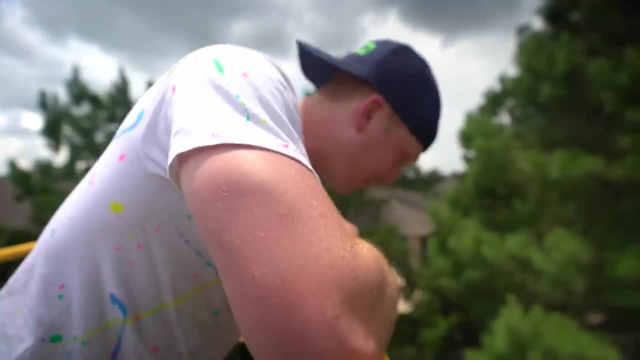 C-U-B-D-A-Q-Q-Q. Three, two, one. Oh man, I would not want to be on the cube. Where'd it go, though The cube? Yeah, The cube probably went through the earth. We dropped the cube and it just goes through the earth and just keeps going. 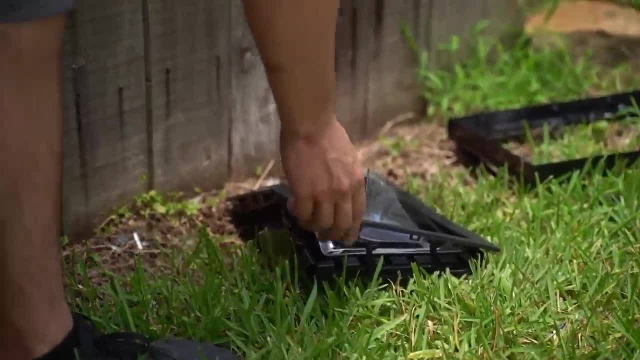 It comes out the other side. Yo, the cube didn't even go through the front screen. It broke it, but it didn't go through. It hit the corner of it. Maybe it hit the middle. There's a metal mesh. It went through metal bro. 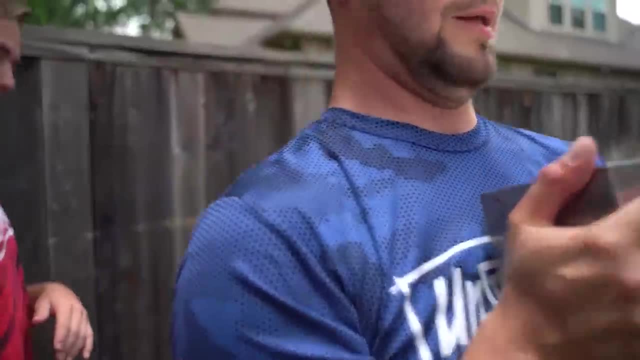 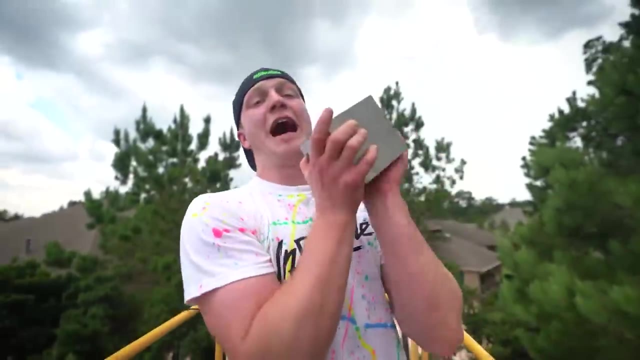 Stop it Metal, All righty. What's our next item? Let me go grab it. Our next item for the indestructible cube is a five-gallon giant thing of water. This is going to be interesting. Now I wanna say I really wanna do a part two to this video, where we try to destroy 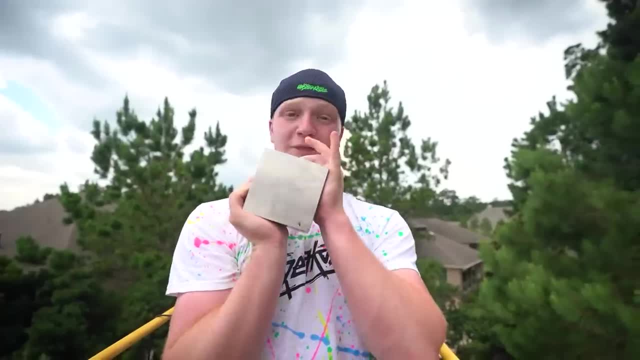 this cube. This cube is more strong than titanium. I wanna see if we can split this thing in half with liquid nitrogen, even lava. If you guys wanna see that, then leave it on the comments. If you guys wanna see that, then leave a like on this video and click that subscribe. 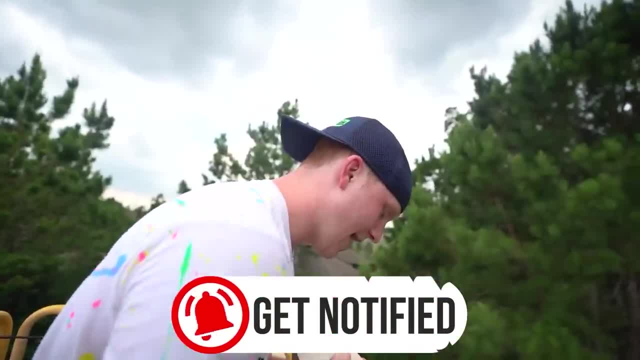 button so you never miss that video. Yo, is that how you want the jug, bro? Yeah, You gonna hit it. I hope so. Okay, Yeah, don't miss, I'm ready for this. This is gonna be like a water park. 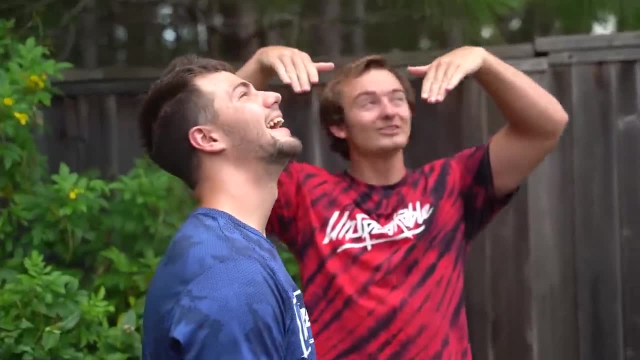 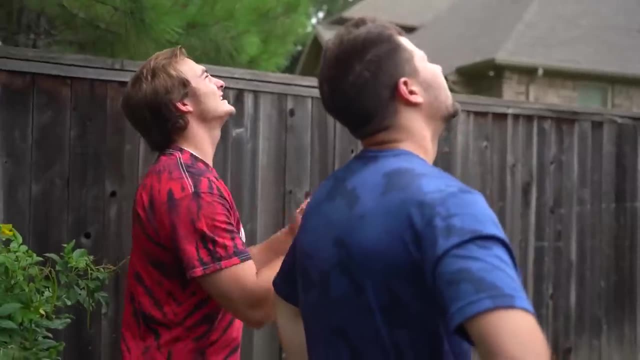 Oh, it's gonna be like you know that bucket that fills up with water and then it dumps on you. I love those things. Drop that cube. Yeah, countdown Ready. All right, Five One, Four, 59.. 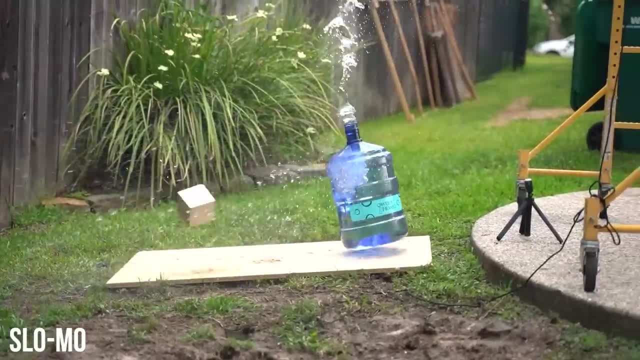 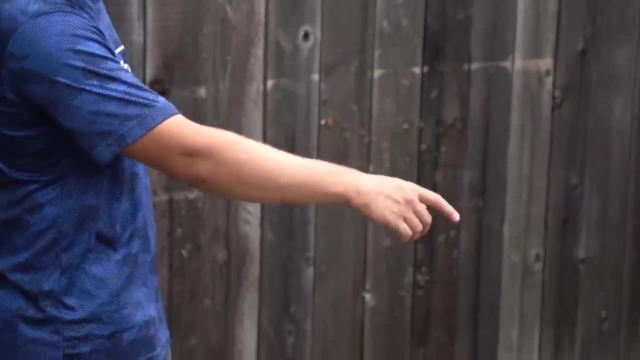 Three, 58.. 56.. Ten, One, Two, Three, Four, Five, Six. Oh, it hit off the bottle cap. That's pretty cool. Oh, look at what it did to the wood. Yo, it broke the wood. 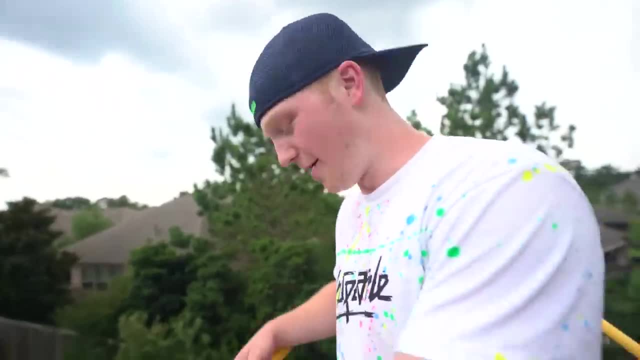 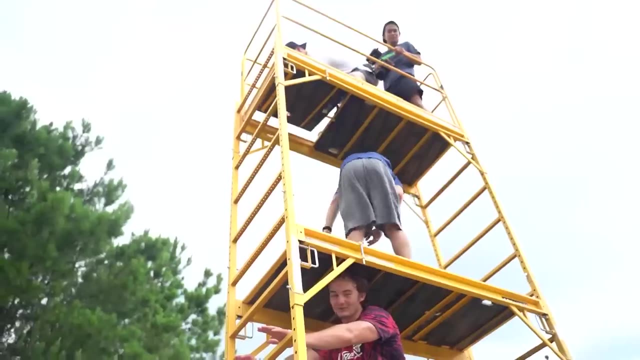 Oh my gosh, That's three fourths inch thick wood. Our genius plan to haul the cube up was great, until it literally went through the bucket. Hi, How are you doing? It's really windy up here. It feels great. It's gonna rain. 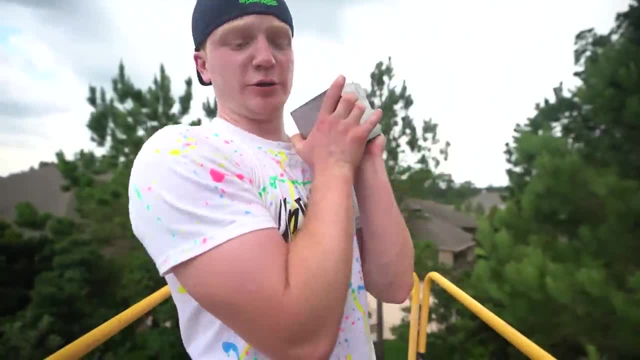 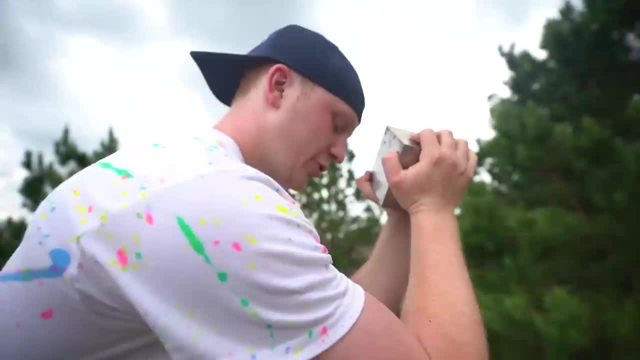 You feel that really cool breeze. All right, Second attempt on the five gallon jug, since we kinda missed the first time. All right, ready. Yo. how's the weather up there, bro? It feels great, It feels nice, Okay, ready. 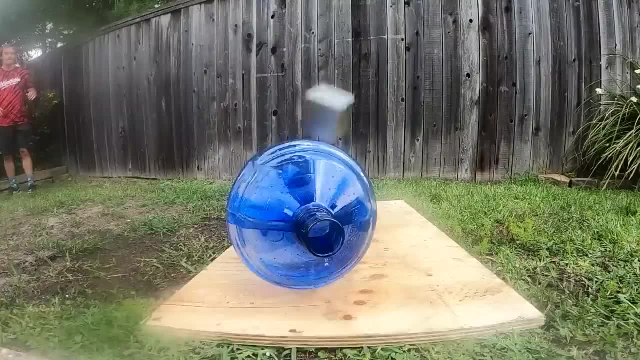 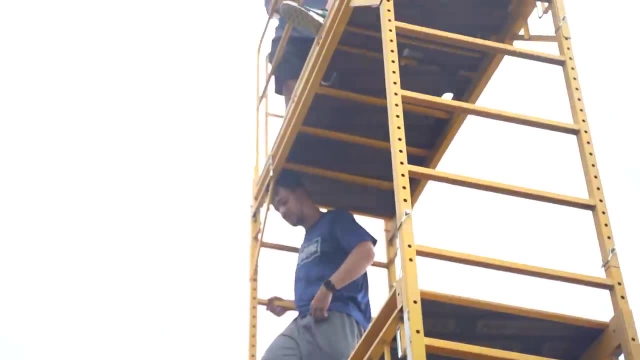 Three Oh Two, It's gonna get water everywhere. One: Oh, I missed. Oh, come on, I missed You gotta hit the thing. It went straight through the wood, All right. now I'm confused: Is the object the wood we're trying to destroy? 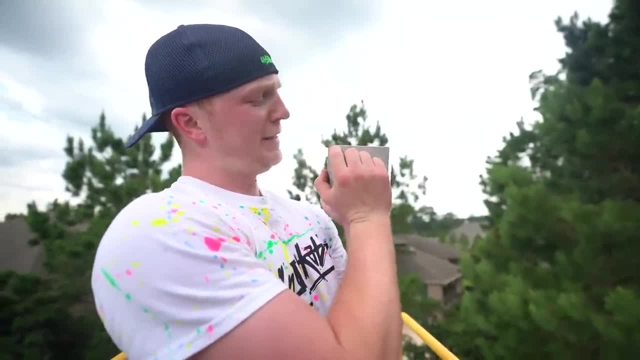 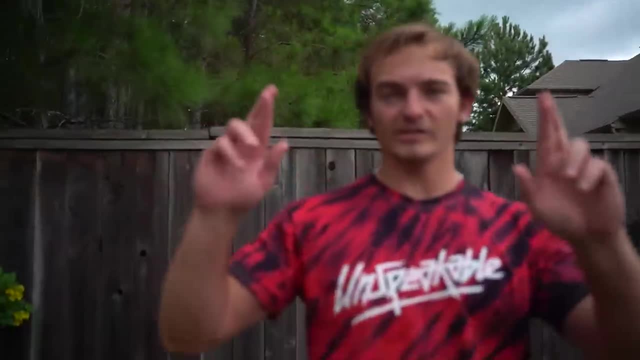 So far, we've dropped the cube a couple times and I see a little little, little tiny scratch right there. You see it right there. That's it. That's it. Hopefully Nathan hits it this time. Cross your fingers, boys and girls, guys and women, men and women, just get this jug. 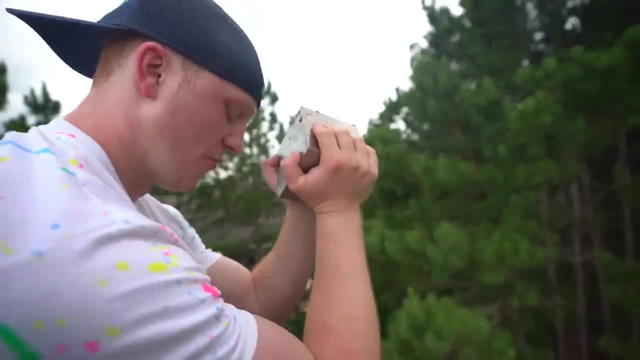 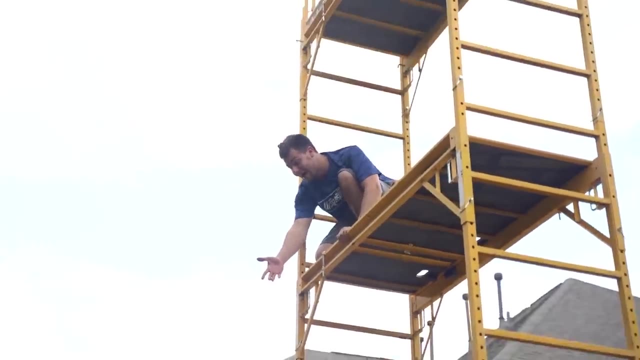 All right, here we go, We're ready. Three, two, Hit it this time. One, Come on. That's the exact same spot. Yo, get off the scaffold. It is a lot harder than you think to throw a 42 pound cube 25 feet down and perfectly. 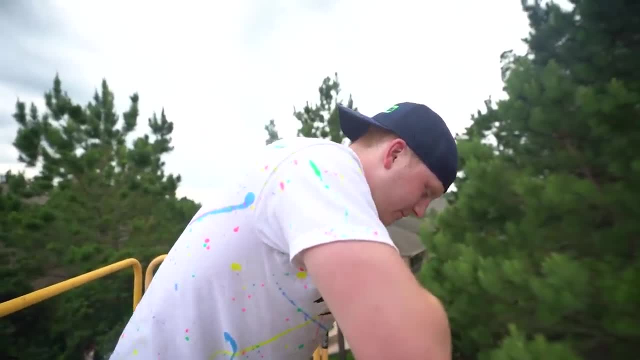 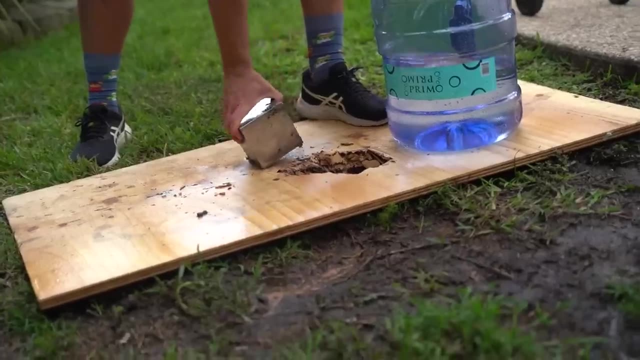 hit an object that looks like this. Should we just move the water jug, this time to where the cube's been laying Ow splinters? Does anyone else want to try? Gabe, go up. Oh gosh, Me and Nathan swapping. 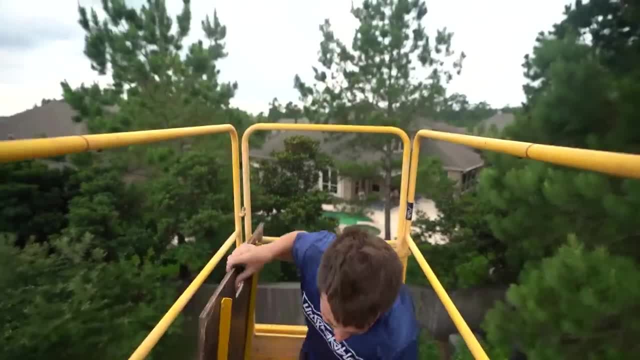 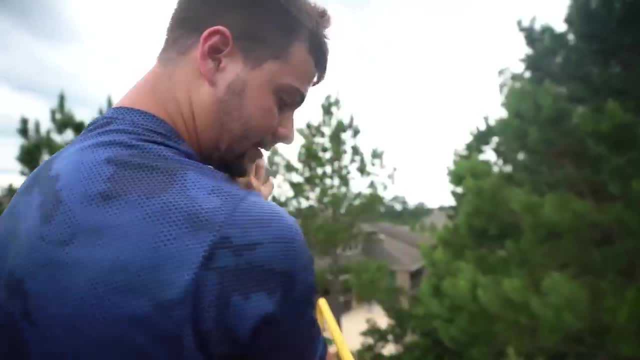 Is that what's going on? Yeah, Okay, I'm the replacement I got it. Don't drop on my thumbs. Let's wait for the cube to be delivered, Is that right? Yes, Go, Okay, Wish me luck. 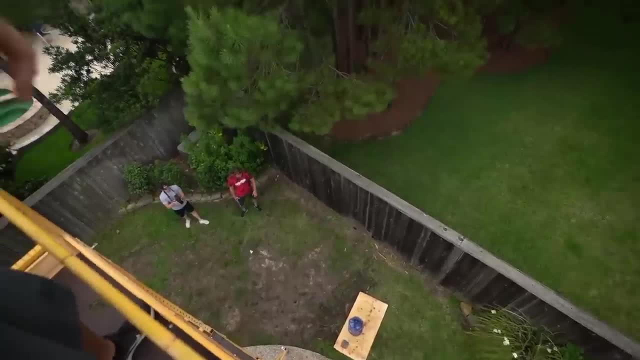 Go for it, Okay, All right. So it's in between me and in between Nathan, All right. Is that a cooking pot? Our next item is a cooking pan. This thing is pretty thick, It's a poncho And it works well. 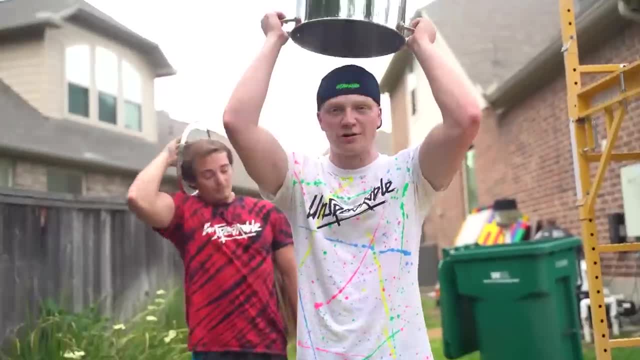 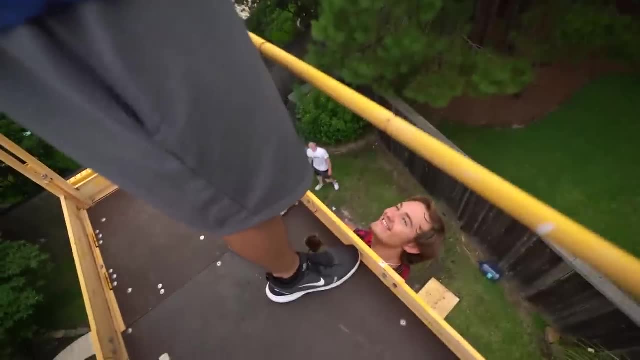 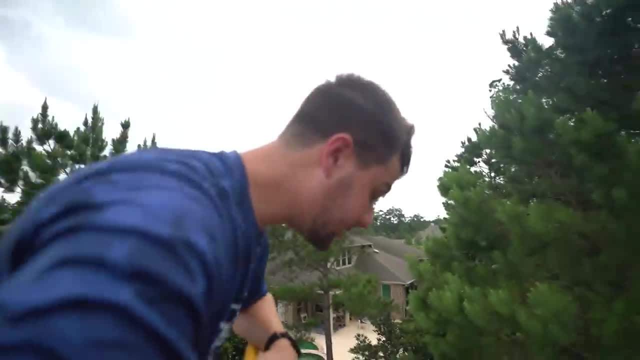 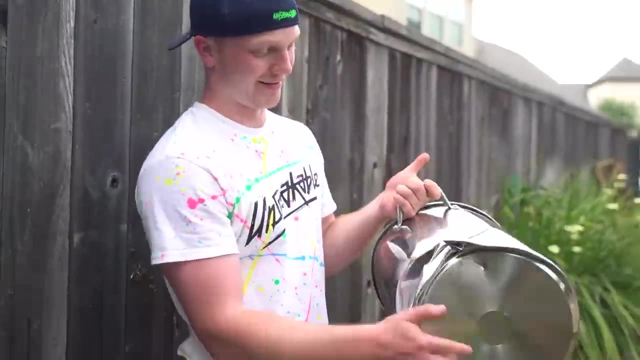 All right, I want to move after that. You ready? I'm ready. I don't know if I am ready, I don't know. This thing goes flying. Here goes Nathan, Here we go. Oh, That did not do as much as I thought it would. 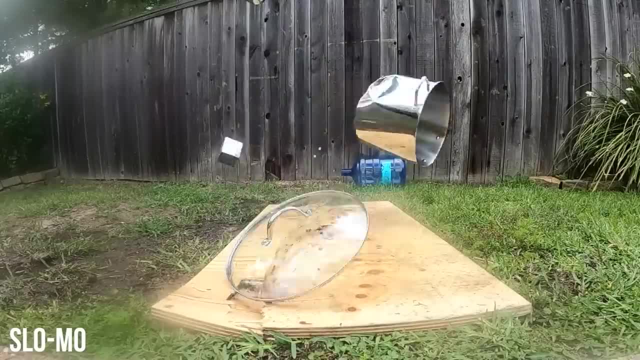 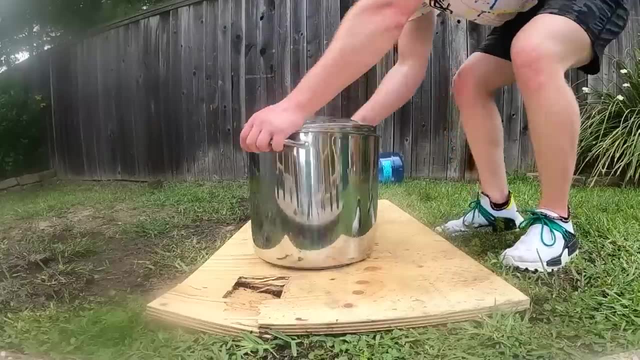 Oh, What I mean? that is steel. Oh snap, You've got to remember. this pan is literally steel And that's pretty impressive. It's not like you missed it either. You hit it pretty solid. Yeah, really fit. anymore sideways would be cool. yeah, i like sideways. okay, second attempt for the steel. 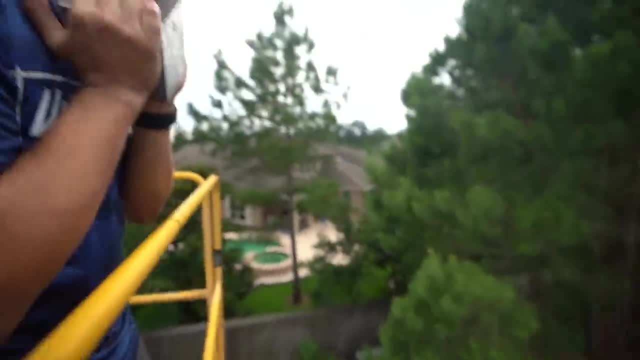 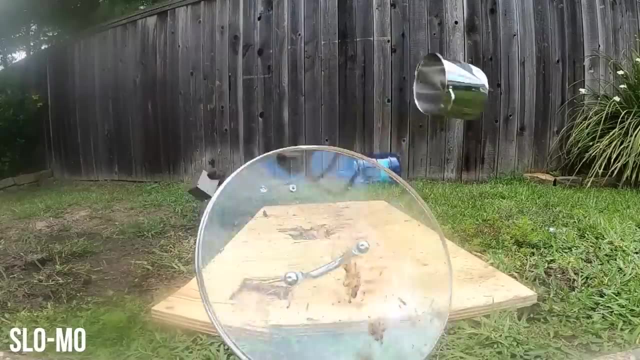 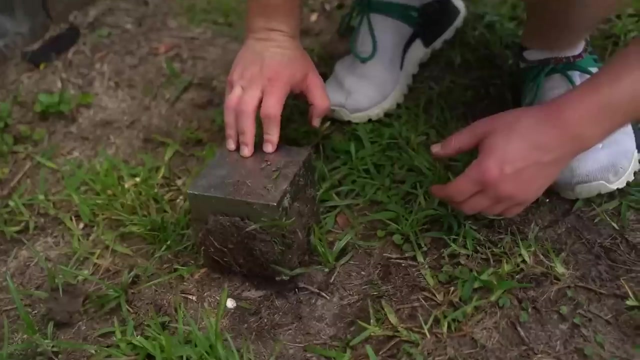 pot. all right, here we go. all right, here it goes. here goes nothing again. i don't know if i should cover my face. oh my gosh, that pot is unbreakable. how's the cube? it's got a big chunk of mud on it. it looks scrumptious, no damage. looks like it got barbecued, all right. next item: stephen wendy's. 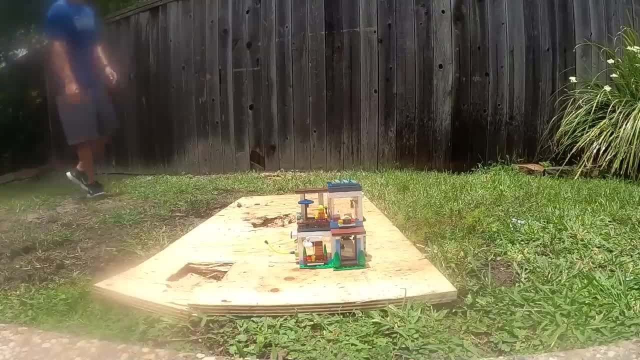 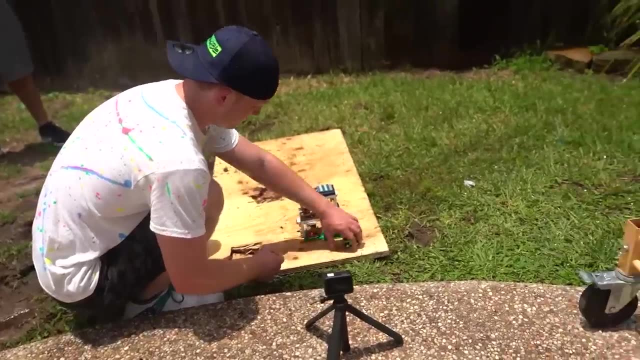 house, bro, who's steven wendy. look at them. oh, they're so happy. steve wendy's inside in her car. there's a car inside. you see that yellow stick. it attaches in front of the car. it's a tesla in front. 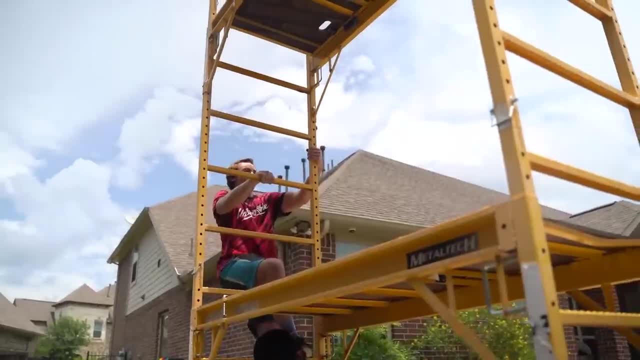 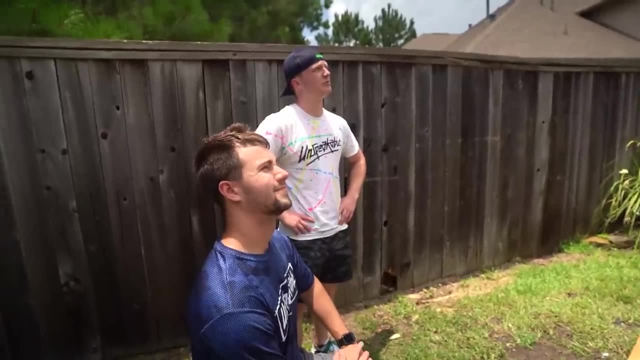 of the car. okay, okay, okay, okay. sorry, you might survive from the meteor strike that's about to happen. oh, the roof comes off. can i just drop it on the gopro instead? no, don't drop it on the gopro, it's worth money. this is a uh sad time for a meteor strike. let it rip with one big meteor. 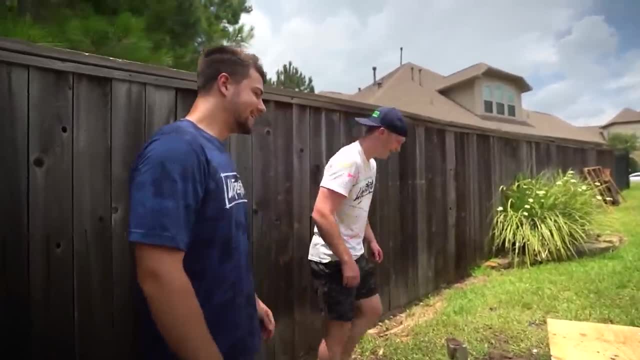 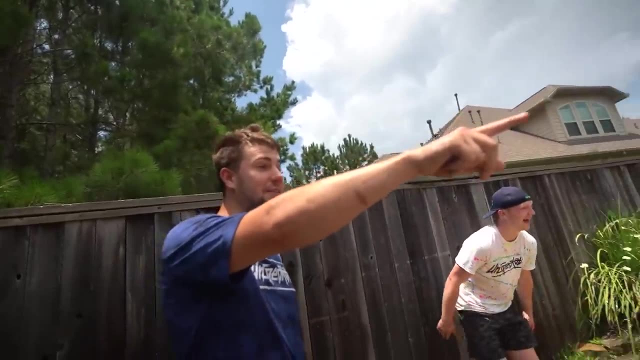 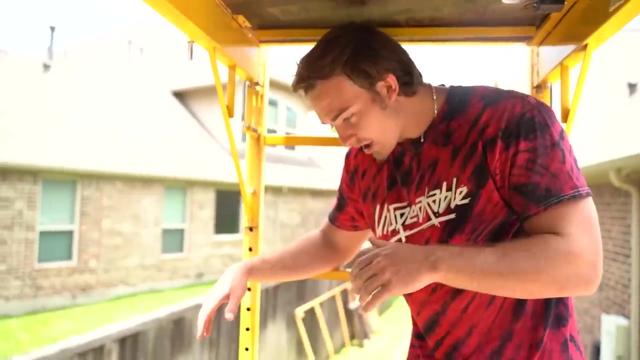 one really, really big meteor. oh, that's pretty cool. wait, it didn't land on her, yo. a piece flew like 30 feet. it went all the way across the board. report unspeakable. he's a murderer. you just killed wendy, at least. okay, look at steve's. 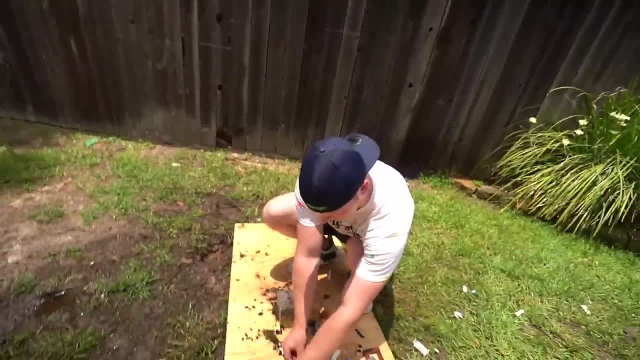 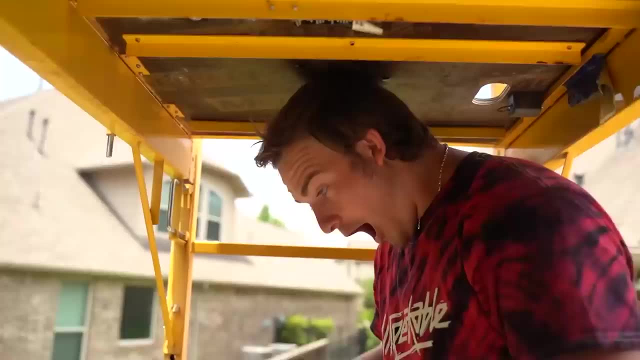 still okay. where's he at this one? no, no, steve, we got steve and we got wendy. oh, that's just messed up. that's just messed up. it would be sad, but that would definitely cool. we gotta wash them off. get off that cube. 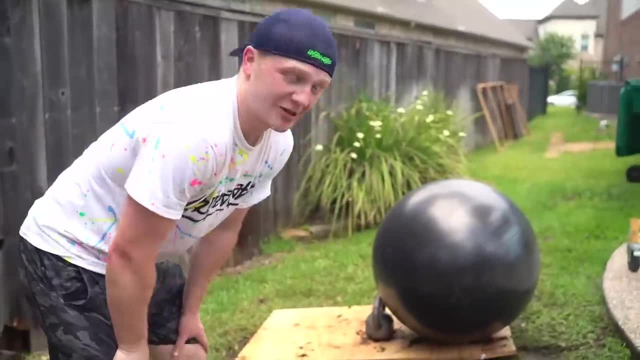 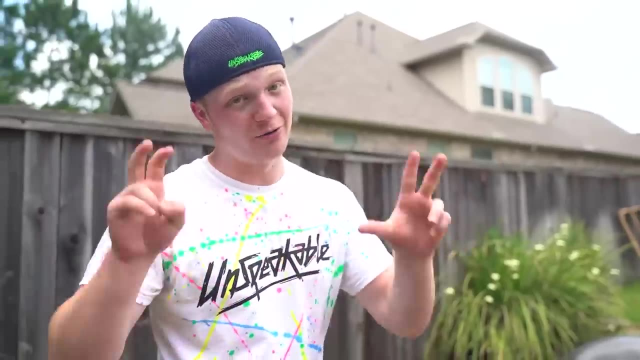 stop, stop, stop, stop. this is our next item that we're dropping it on. this is gonna be interesting, because this yoga ball, or medicine ball, is actually really, really tough. i can't wait to drop this cube. apparently, you can cut this thing with a knife and it won't even pop, not like completely. 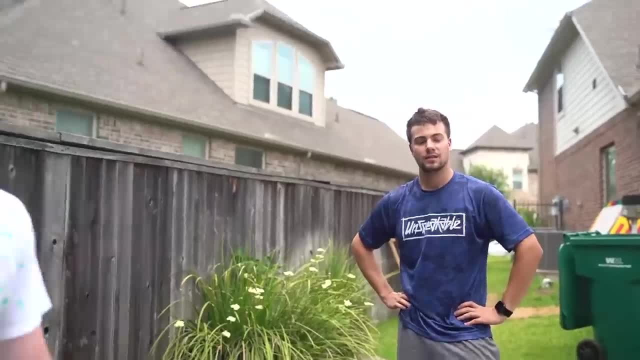 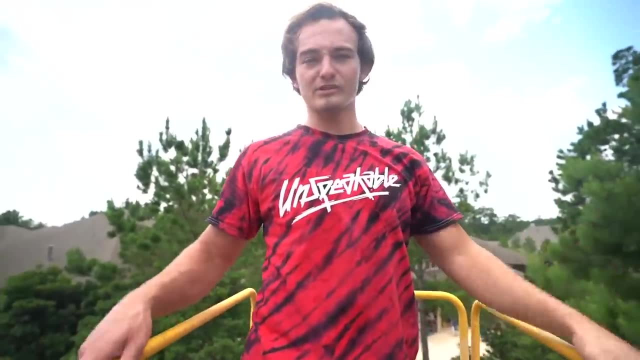 but like just a little, you know little incision. anyways, I really think that this cube might bounce off. I really want to miss it on purpose, Cause like they both suck at dropping this cube, I hope it bounces off, but then I'm really scared. 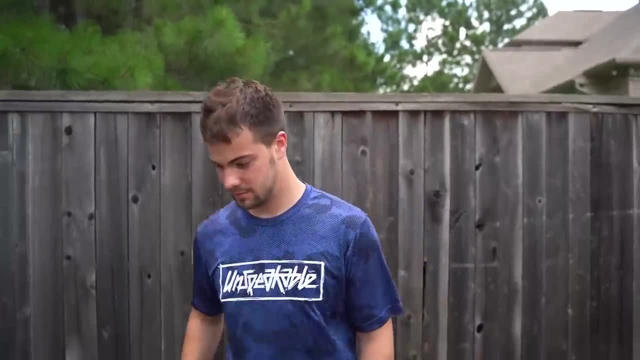 Let's just take cover, okay. Yeah, I will be behind that wall over there. Let's just take some cover, dude. All right, you ready? All right, I'm ready. I'm also ready to run if it bounces this way. 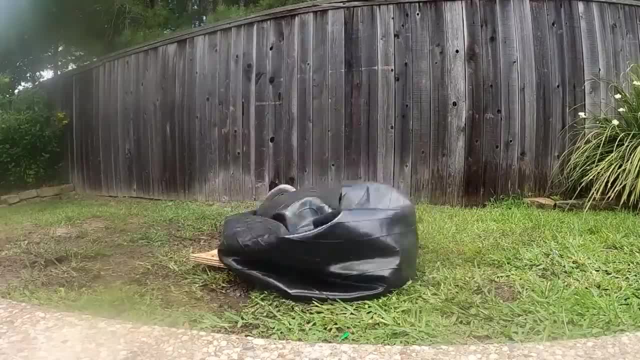 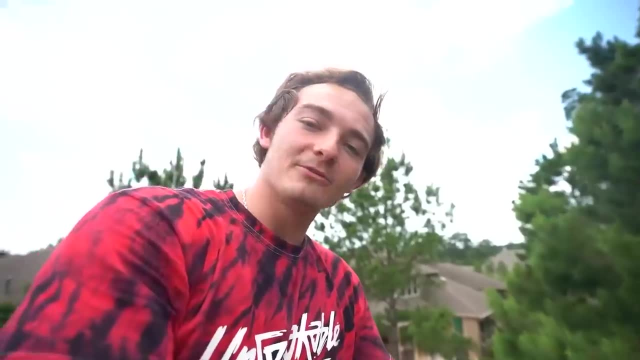 Three, two, one. Oh Oh, I thought it was gonna bounce for a second. That's where I said it was gonna happen. I'm so sorry, It just went straight through the wall. Wow, it bounced so high guys. 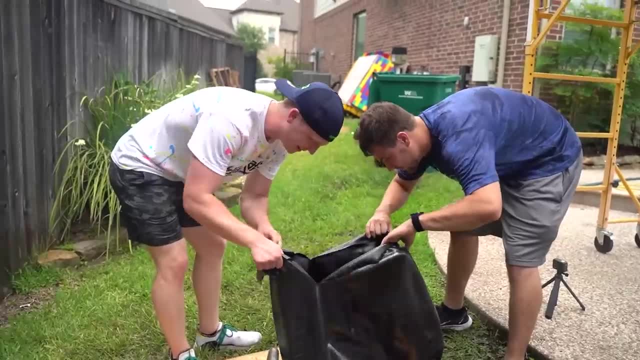 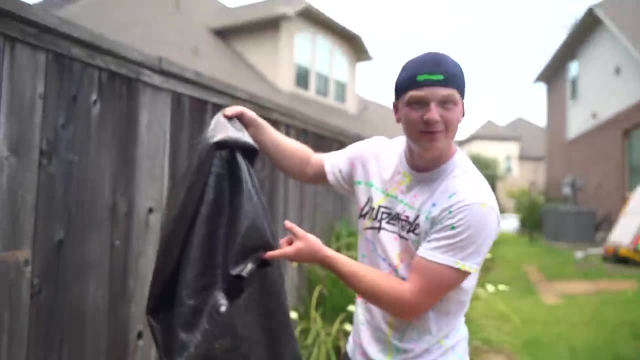 I know You guys have no faith in my college degree. Where is the cube? Oh, here it is. Look it's right here, Found it. There's the cube. Oh my gosh dude. Oh, it went through the other side too. 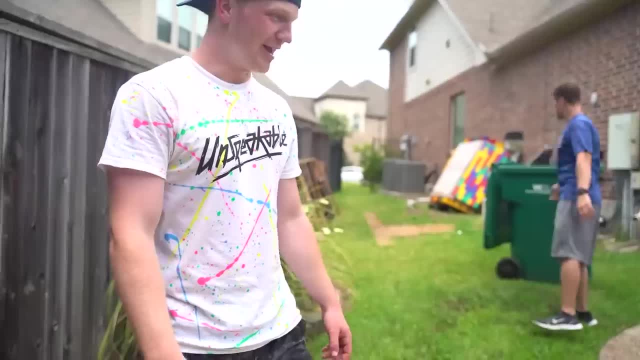 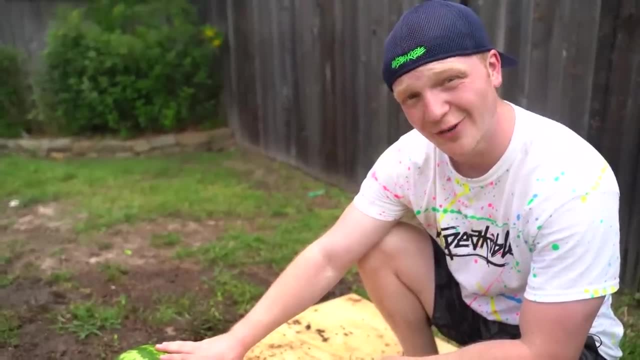 That is insane. Honestly, not surprised it did that. Next item, Next item, All right, our next one is this beautiful watermelon. It is beautiful And we're gonna see what happens when you, you know, drop an indestructible cube on it. 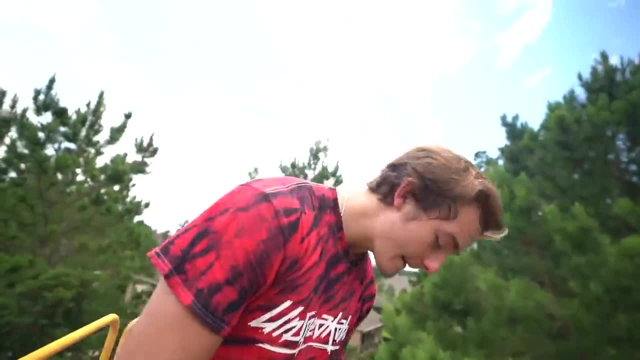 I don't think it's gonna make it. No, it's definitely Good luck. Good luck, buddy. You ready, Are you ready? I was born ready. Drop that cube. Three, two. Oh, I'm gonna miss this Hardcore. 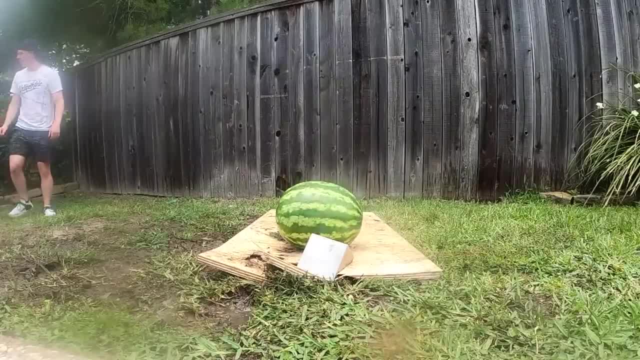 Three, two, one. Yeah, I knew it. Oh, and we have a miss hit. I knew I was gonna miss it. It was too far away. You know how they all complain on how it's too far, It was too far. 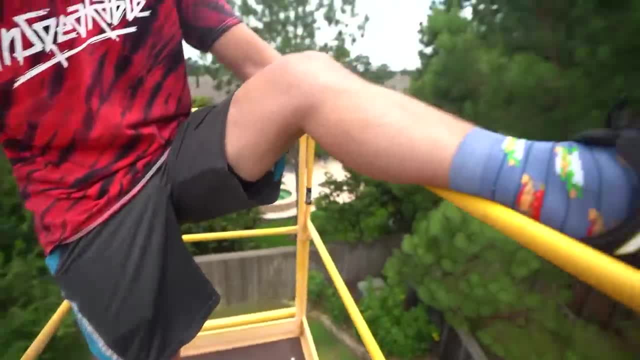 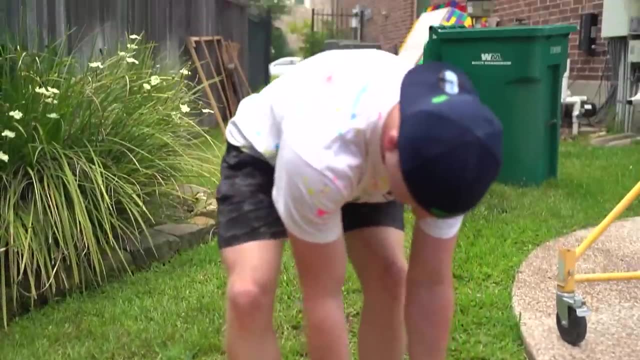 I didn't complain because I'm a man with Mario socks on Man. that wood is getting destroyed. Oh my gosh, dude. All right round two. Hopefully we hit the watermelon. Let's hit the watermelon this time. 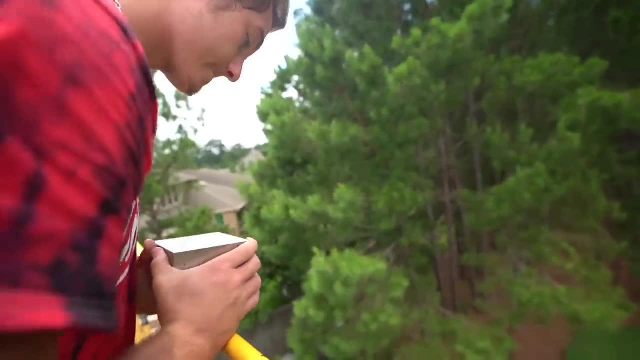 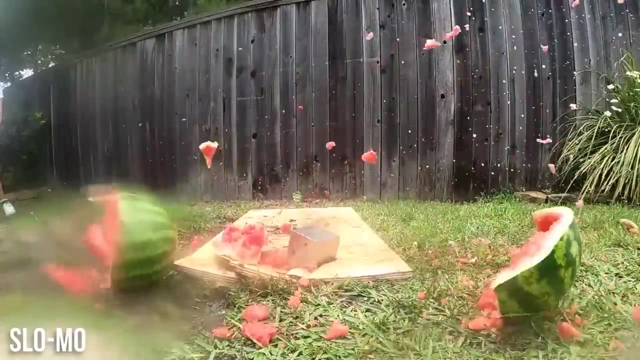 Goodbye, watermelon. Hope you had a nice time at the grocery store. I bet you didn't know you were gonna get bought by a YouTuber. Oh man, that exploded. Well, that's one way to open a watermelon. 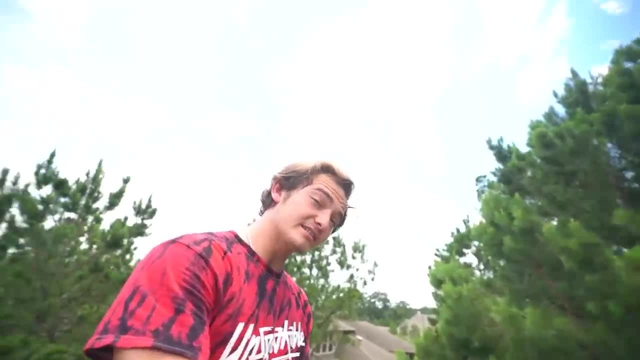 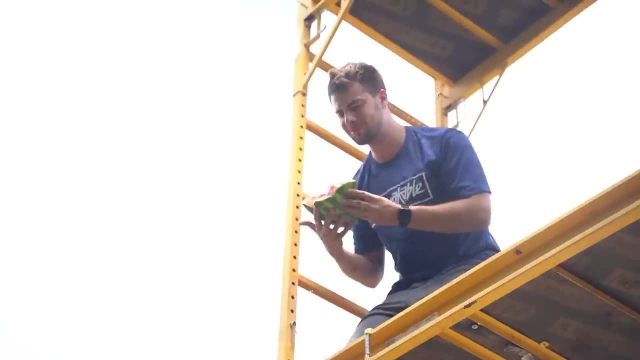 See if it tastes good. Yeah, let me see if it tastes. all right, I bet that watermelon tastes good on this nice hot summer day. Perfect, Pass it on up. Here you go. What a throw. Yo pass it on up. 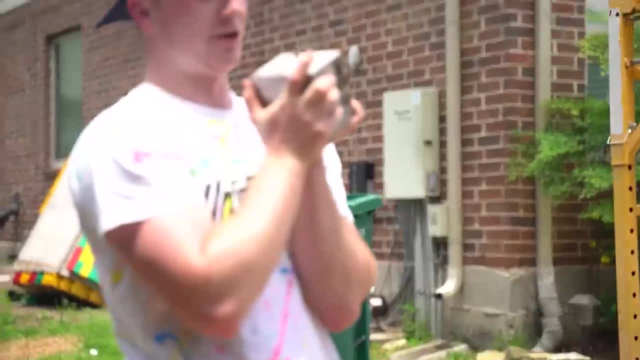 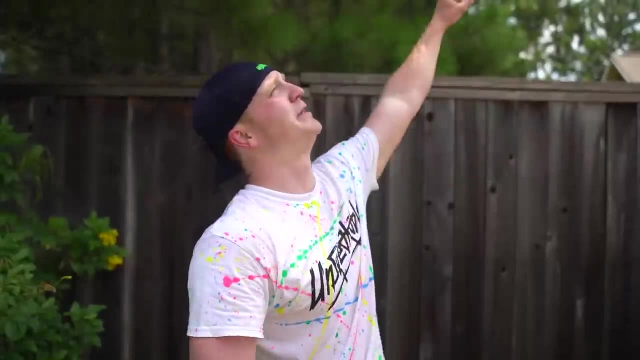 That's pretty good. It's not Super sweet, but it's good. And so far, damage to the cube: nothing At all, Not a single scratch, As Buzz Lightyear might say, to infinity and beyond. All right ready. 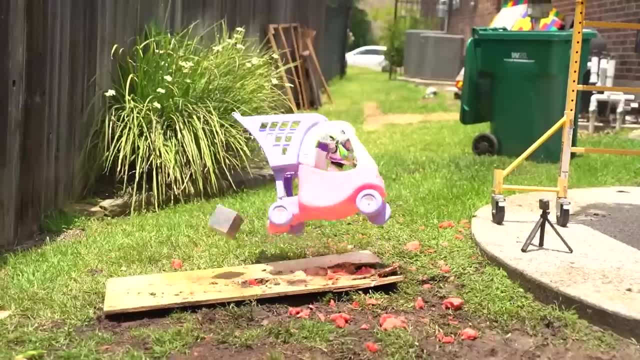 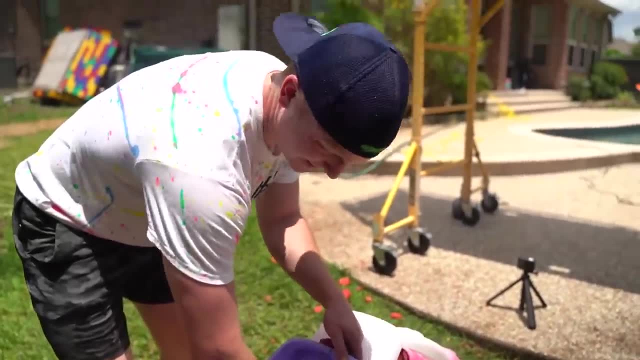 Buzz Lightyear Three, two, one Did not sign up for this, Bro. did I even hit it? It literally just went straight through right here, Zero resistance, As you can see, But we're gonna try to land right here. 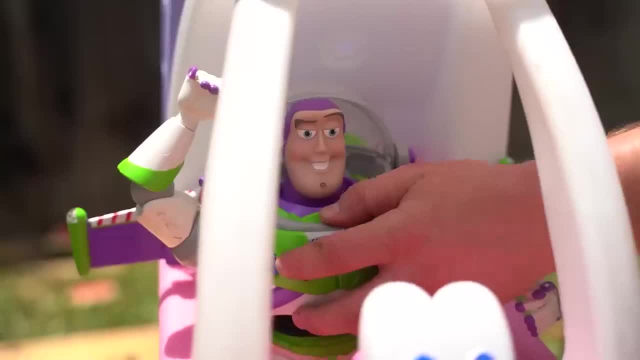 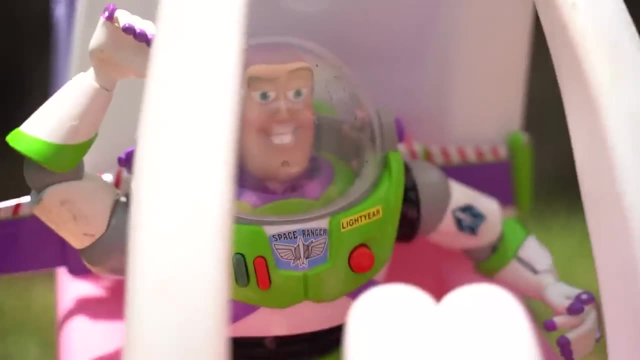 Let's get Buzz Lightyear back in there. I'm sorry, buddy, You did not ask for this Laser in full power Approaching destination. Buzz Lightyear is at your service. All right, buddy, you're gonna have to put that boy down. 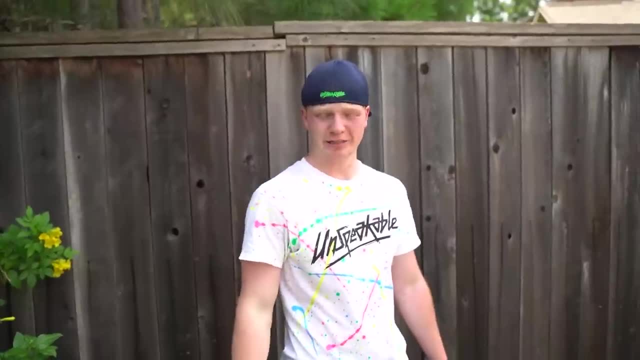 because it's about to get serious. That is a sweaty day. I'm out here sweating for you guys, dropping a heavy cube, hauling it up there. You guys gotta leave a like on this video, especially if you want to see us try and attempt. 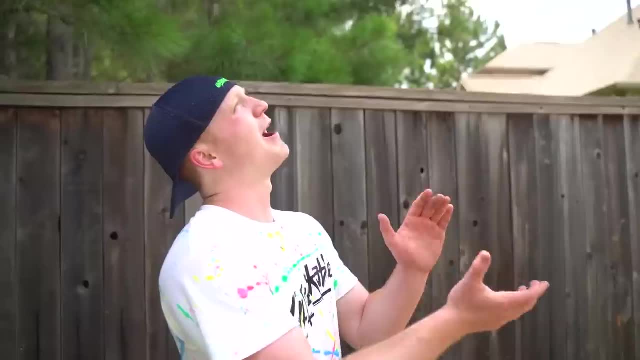 to destroy this cube with lava and liquid nitrogen. So leave a like. All right, you ready, I'm ready, let's do it All right. three, two, one, To infinity and beyond. Oh, you lost a leg. 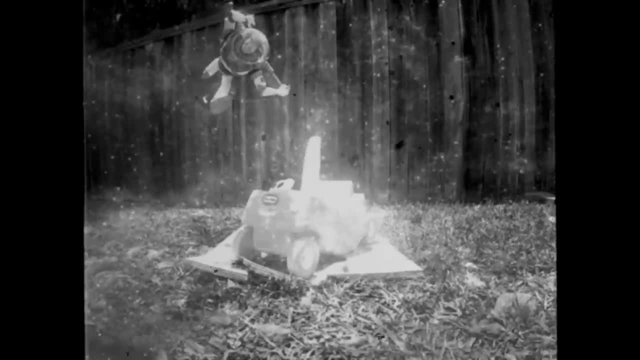 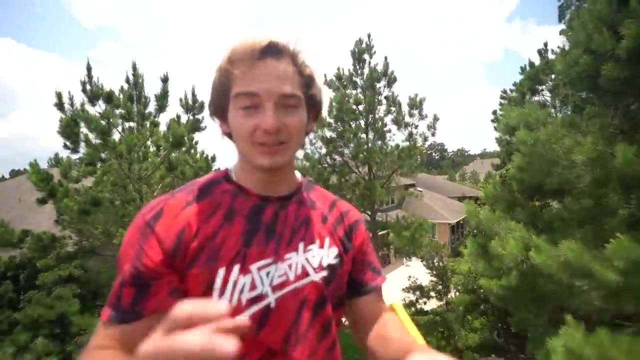 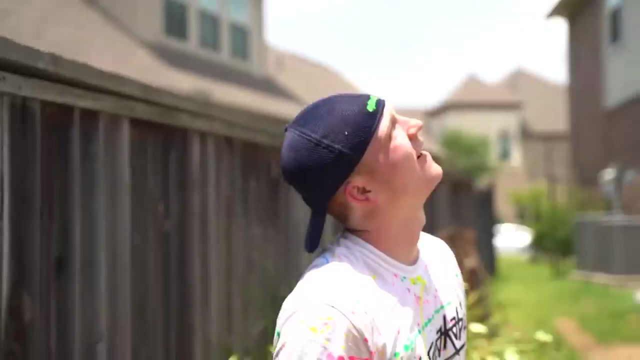 Approaching destination, re-inducing gravity. Buzz Lightyear is at your service. Oh, it looked like he was coming to fly up to us. Oh, it's his leg, the one he signed. Get the cube out of there, All right. next. 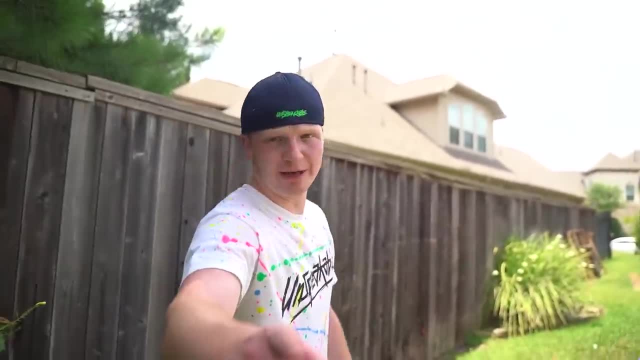 Next item: we have a big gallon jug of paint- Blue paint, Blue paint, to be exact, Blue paint. All right, you ready? Maybe it'll make your shirt more tie-dye. Yeah, it might make my shirt pretty. 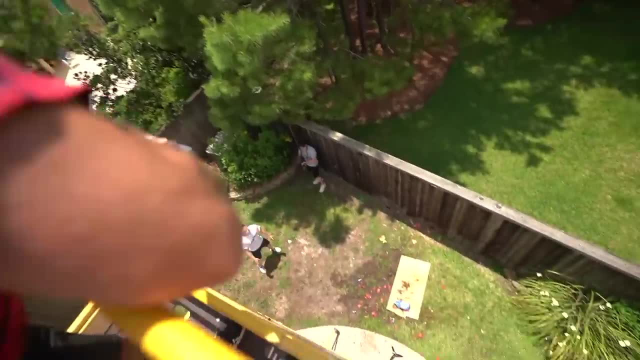 Yeah, get a little closer to it. All right, I want to stand right here. All right, three, two one. Three, two one. Oh jeez, That worked so well. Yo, I got some of my arms. 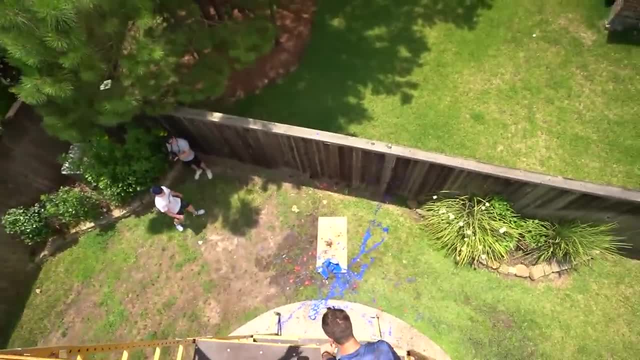 There's blue paint everywhere. There's some on the top of the fence, Like all over the ground on the fence. Oh my gosh, It even shot up on the first floor of the scaffold. Look at this, look at this. come here. 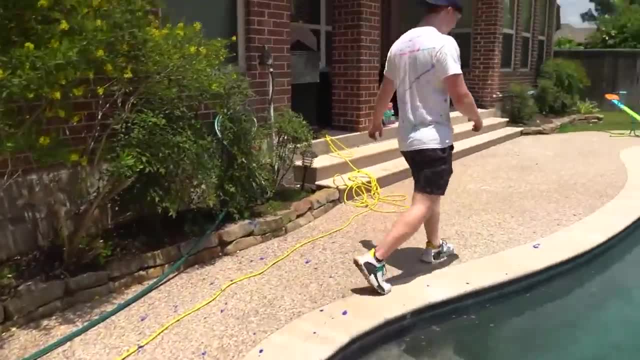 It goes all the way over here. look at that. All the way across the pool. Yo, where's the tape measure? All the way over here, across the pool. This right here is my beautiful creation, just a little pyramid. What is it? 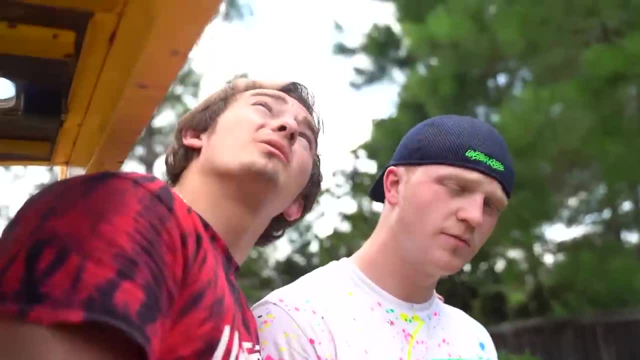 What do you mean? what does it look like? Well, if it's your beautiful creation, you could go, uh, Go up this scaffold and destroy it. I would love to, actually, I would. I would absolutely love to do that. 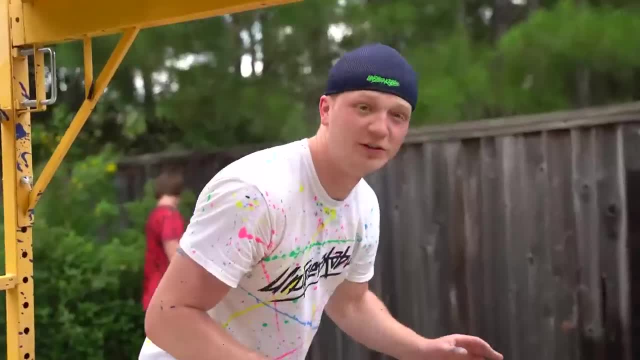 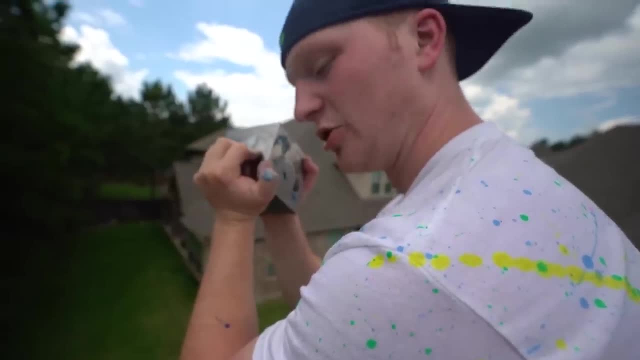 I'm going to give him a little bit more. Let's go drop a insanely heavy cube on this super light cup tower. Dropping the indestructible cube on a solo cup pyramid tower. Here we go. Three, two, one. Whoa, that was pretty cool. 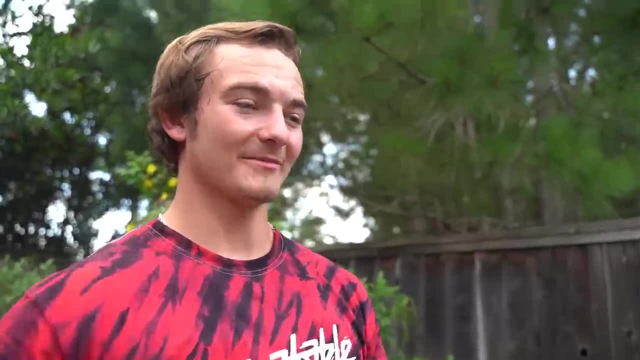 That went way better than I expected, honestly. Oh, there was a cup that landed. That's all you cared about. That's what I was looking for. I was like these cups are going to flip and I hope one of them lands. 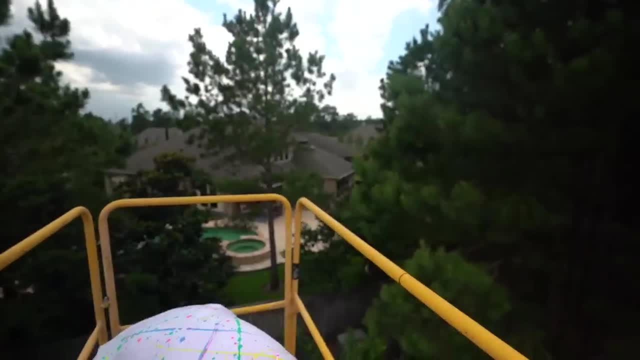 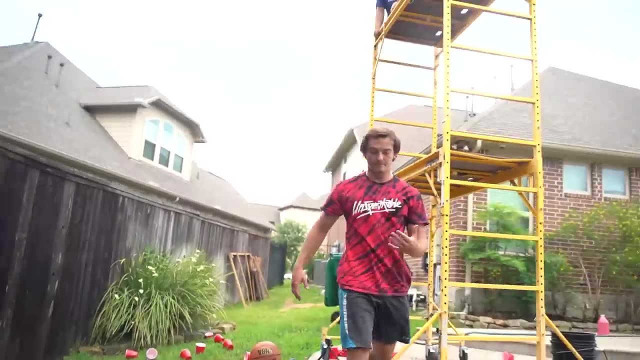 We got three landed upright in the grass. Okay, so for our next item of destruction for the cube is a basketball that is fully inflated. This is going to be interesting Ready, Yeah, Tomston. Cube versus basketball- The basketball is in the drop zone. 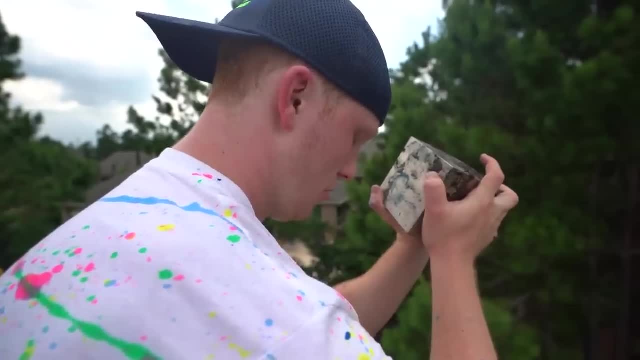 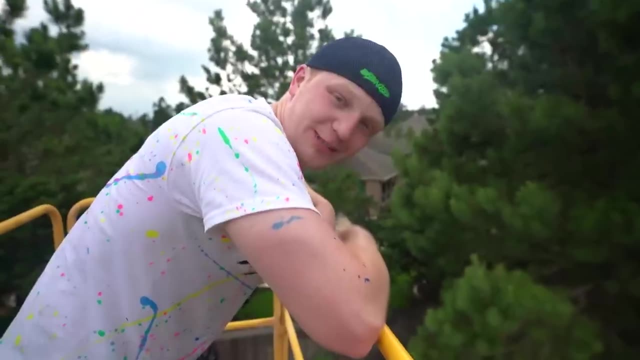 Hit it first, strike. Here we go. Three, two, one. Oh it's gone. It went over the fence, It's gone. We're going to try the basketball again, Since I slightly missed it. it's going to cause it to literally fly over. 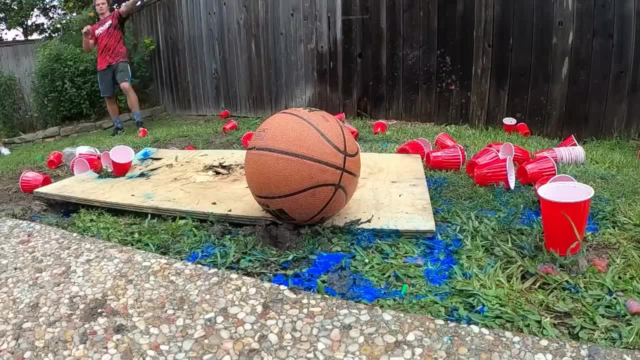 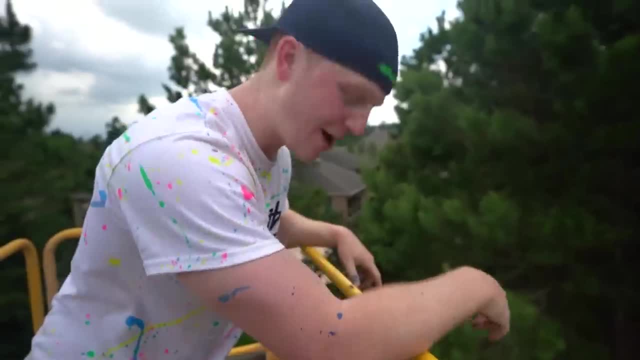 All right. Tip number two: with the basketball. Here we go: Three, two, one, Oh no way, Dude What. It landed right on the basketball and it bounced off. I think we might have found something that we can destruct. 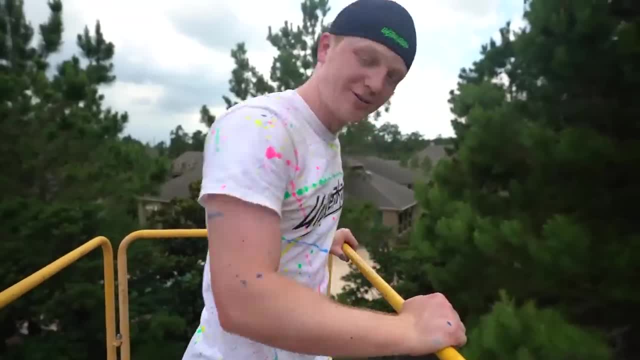 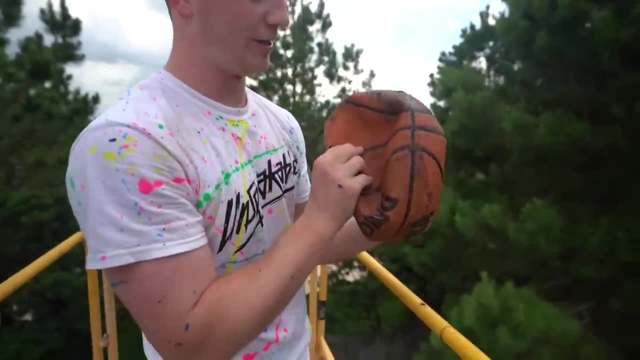 Oh, nevermind, There's a hole in it, Three holes in it, Three holes in the basketball. Good job, Okay, so we got one tear right here. As you can see, this thing was fully inflated before. One tear right there. 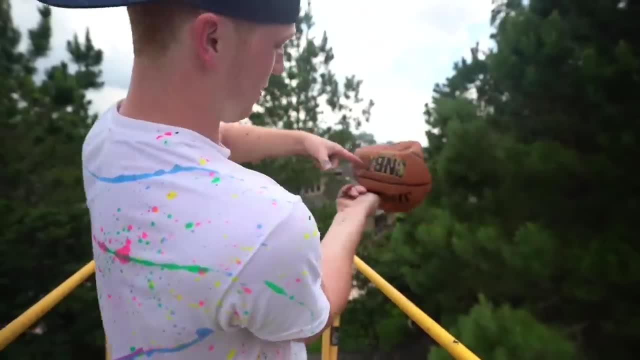 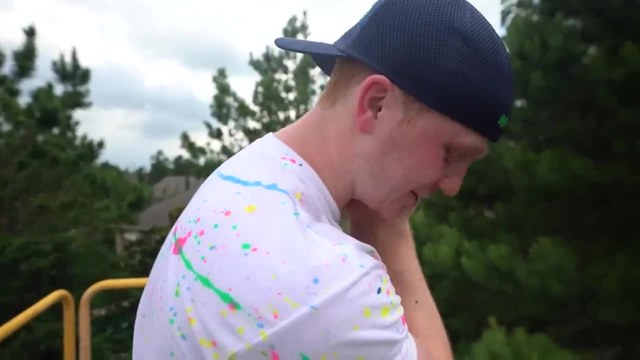 Another tear right there. It's big enough to stick my finger through it. And then another tear back here. Wow, That basketball launched that cube. What is that? like 12 feet. So this is our last item. It is a little tricycle. 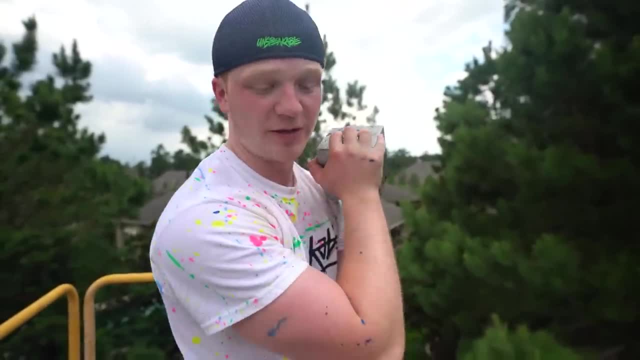 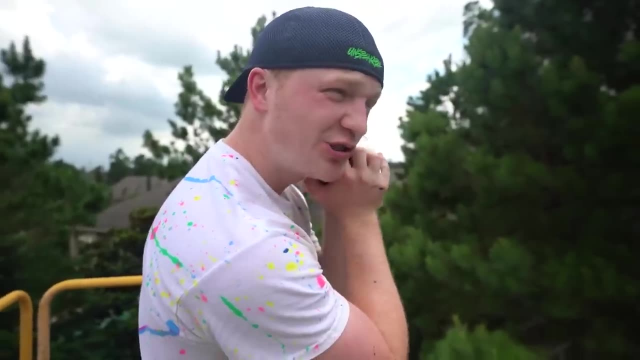 Now, if you want to see a part two, where we try to drop this cube off of something that is twice this height, let us know what you want to see it land on. Maybe we could do a car, Maybe we could do a house. 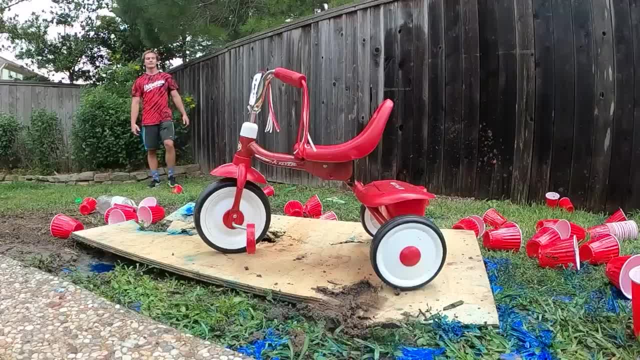 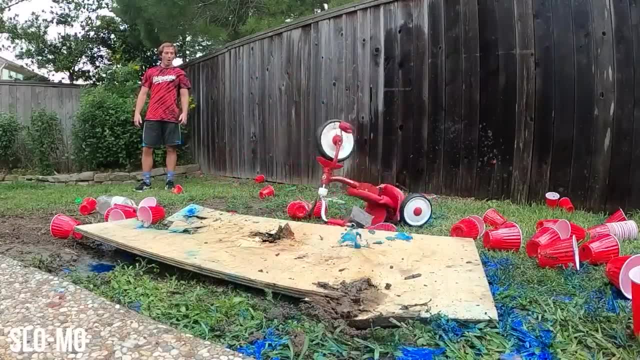 I don't know, Just let us know in the comment section below. All right, here we go. Three, two, one, Not my tricycle, It took it pretty well. The tricycle axle is bent completely. Yo, it's a low rider. 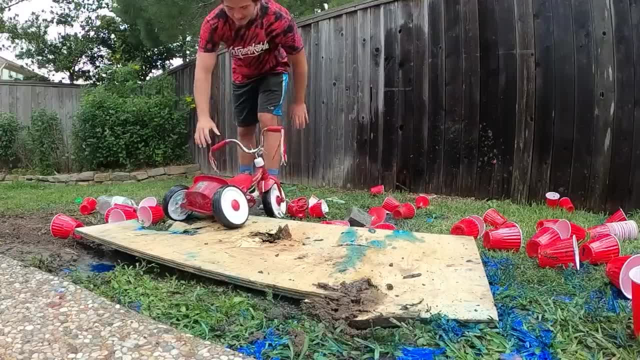 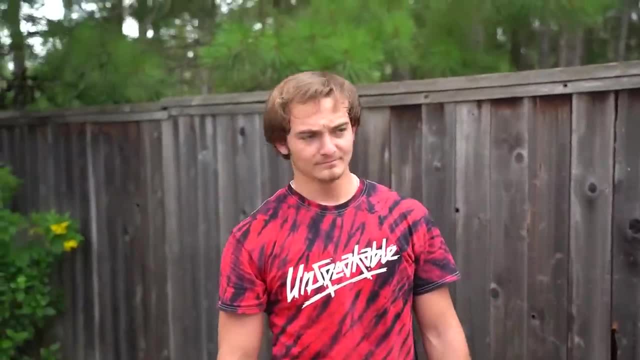 Yeah, Okay, that thing is pretty much done, for I will say: The wheels ain't turning on that one, I don't think it works anymore. Oh my gosh, Poor thing. That's terrible. It served us well, Very well. 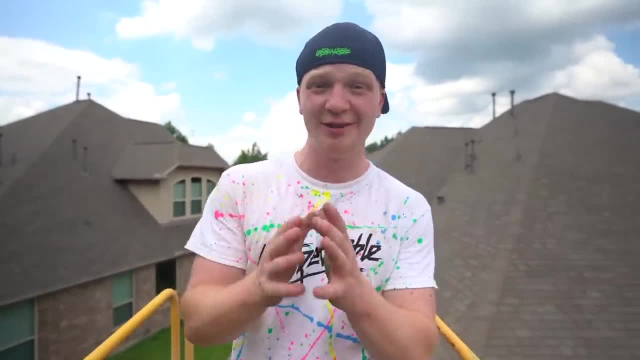 That cube is insane. If you guys want to see another part where we try to destroy it, I want to see if we can break that thing in half. I want to see what's inside the middle of it. Ooh, ooh, ooh. 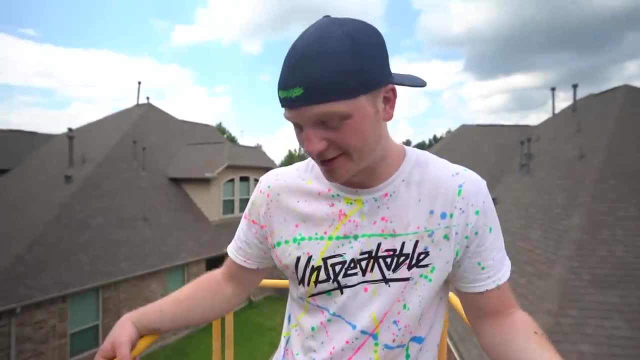 What I got? an idea, Huh, Sledgehammer, A sledgehammer. Yeah, I don't think a sledgehammer is good, Dude, we're going to need like lava, Ooh, ooh, We have a furnace. 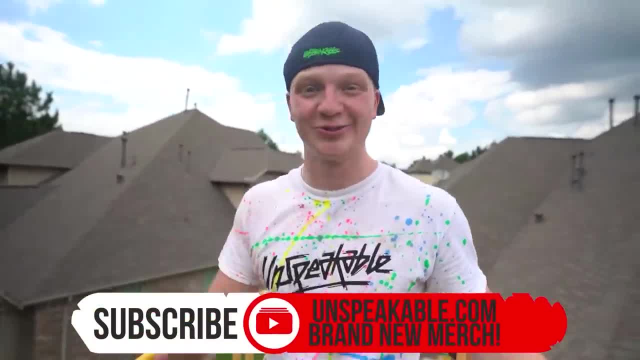 I like it. I like it. So if you guys want to see a part two where we try to destroy the indestructible cube, leave a like on this video. Until then, we'll see you next time. And if you ever want to check out some of the new merch, 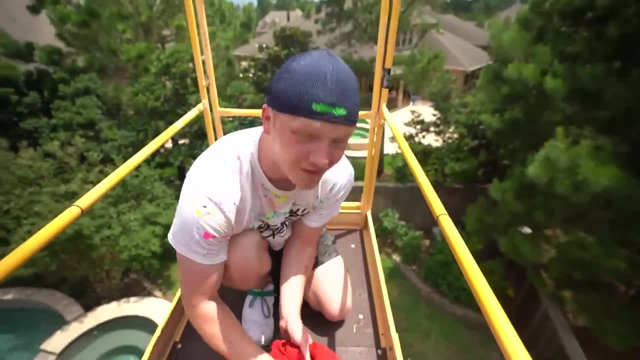 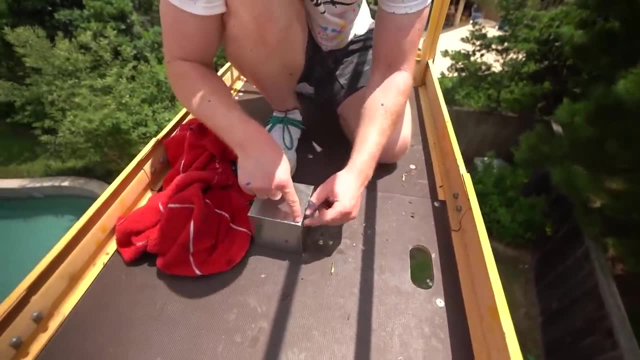 it's right here. Okay so, getting the cube all pretty and check out the damage After dropping this cube on so many different things, look at it, It is literally spotless. There's a little little tiny chip right there, But I mean, look at this thing. 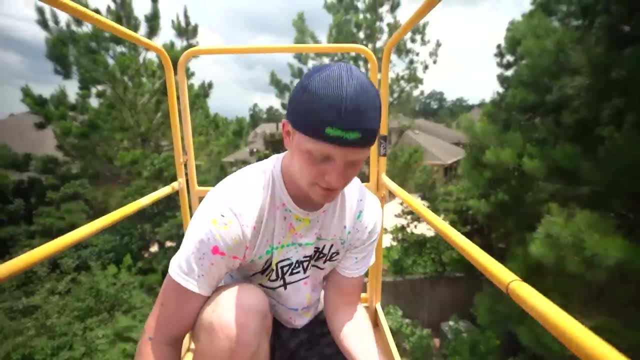 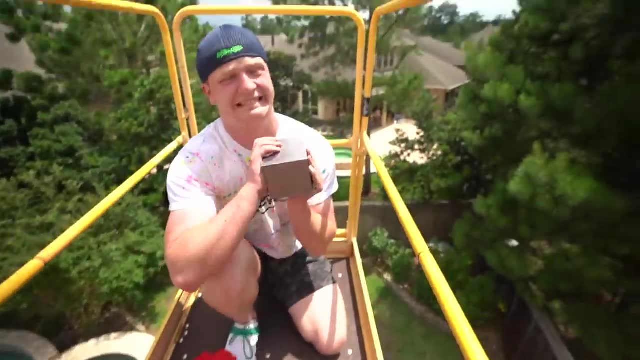 A couple scratches here and there, A little bit of dirt. It's literally indestructible, Like there. there is no damage. That is insane. Are you kidding me? Incredible. It's so heavy I can barely hold it with one hand.